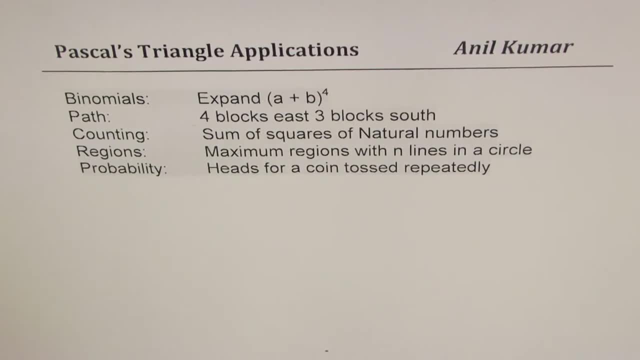 in which each term is the sum of the two terms above it. Now, what do I mean by that? So let me show you. Let's say we begin by the number one. As we move down, we are going, we have two directions to go And then every time we'll go into two directions and rewrite the. 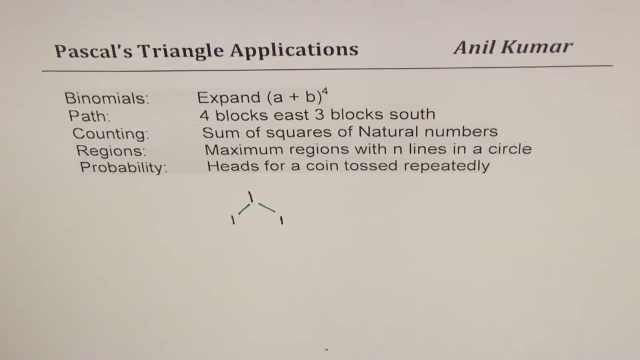 number one: As we move down, we go like this, So these are treated as paths, right? So if I'm here, I have two options: I could go in the same direction, like this, diagonally, or in that direction. So that is how I'm moving, right. So as I move, I'll be placing one on the side. 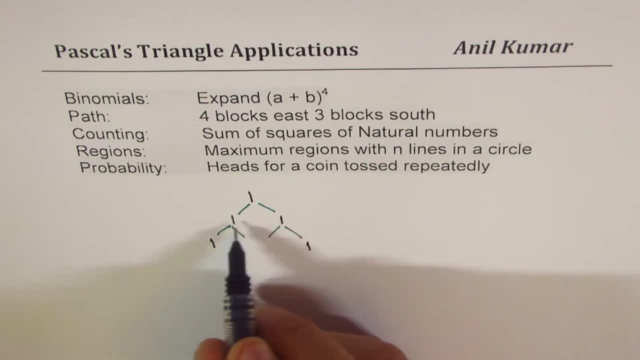 and the numbers which we come in the center are some of the numbers above it. So one plus one is two, so I'll place two here, right. So that is how we build Pascal's triangle. So let's just build it up. 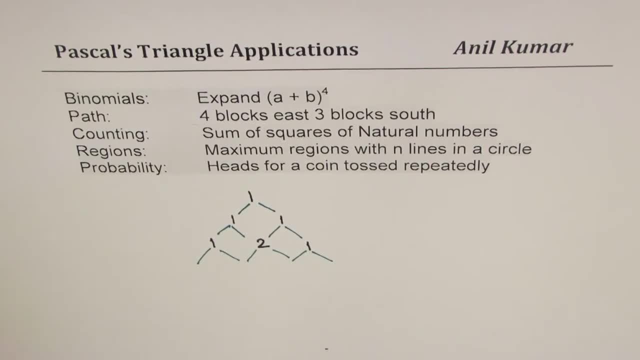 And you will soon understand its importance also. So on the left and the right wings you can say: keep on getting ones Inside. add the numbers: One plus two is three, Two plus one is three, correct. Now let's make few more, And then we'll take up examples. 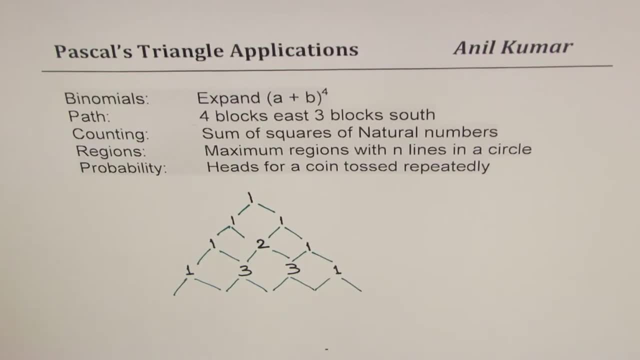 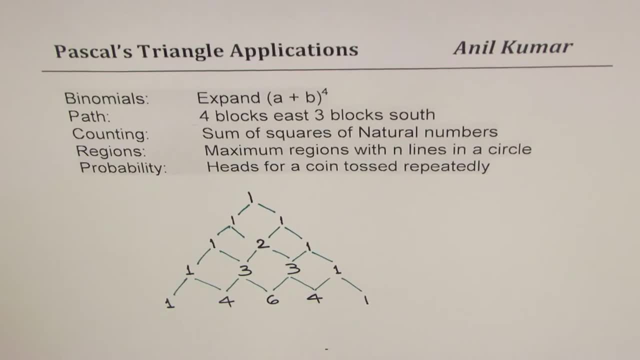 plus three is four, and this is one. Let's go one more time right. So now we are on the fifth row. So when I get five, I'm on the fifth row. If I get to six in this position, it'll be the sixth row, right. So one, four plus one is five. Six plus four is ten Ten. 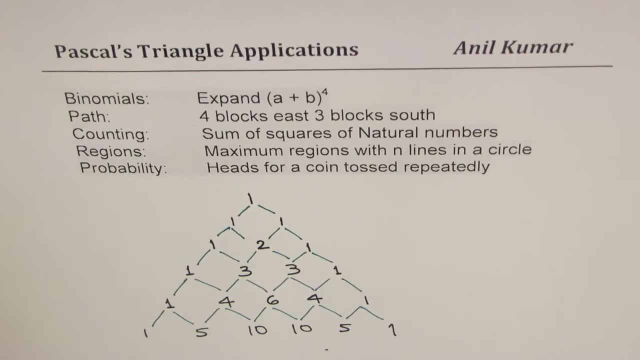 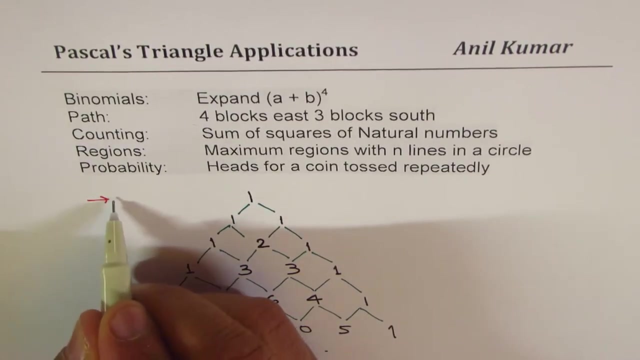 Four plus one is five and this is one correct. So what we were seeing here is a Pascal's triangle. right now, we normally will always refer the first one as not one. this we refer by the name of rows. we call this as zeroth row, right. so row number zero and the next one is number one row is that? 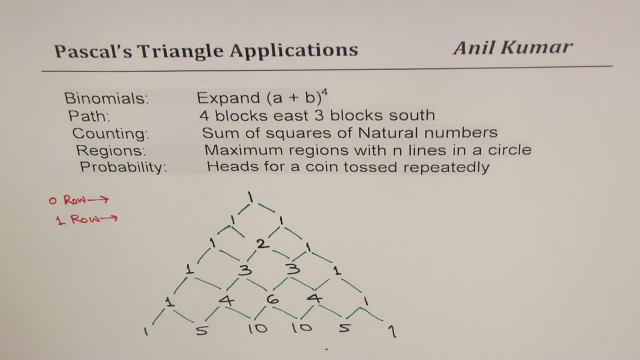 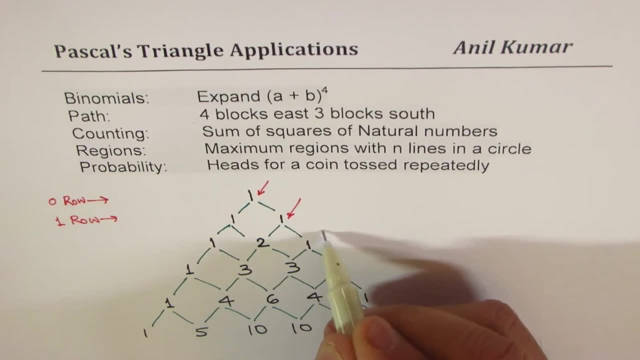 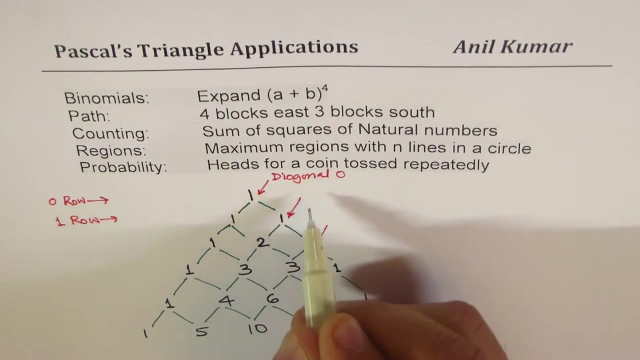 okay, so that is how we are treating each term here. so we talk about rows and these are called diagonals. right? so these are diagonals for us and just as we named rows, we'll name diagonals as diagonal zero. this is diagonal one and this is diagonal. 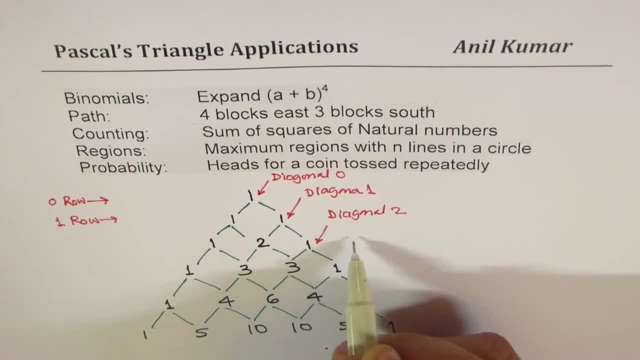 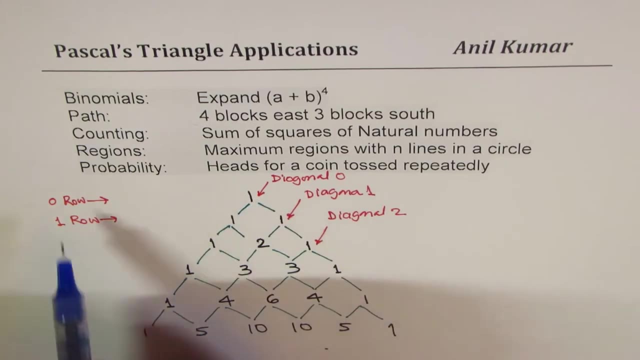 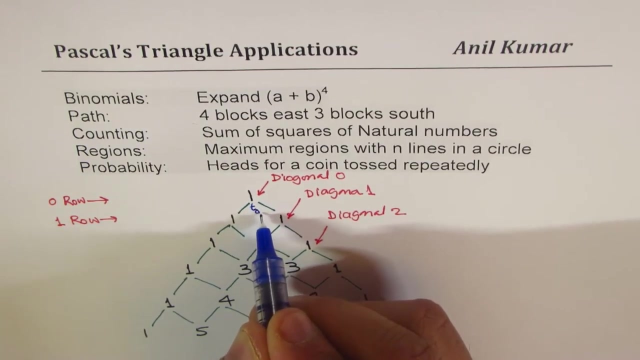 two and so on. so these are the diagonals for you and those are the rows for you. so we use term numbers to identify each and every position here. so this position here will be treated as row zero, diagonal zero. t for term right. so we'll write this as- let me write small t- zero, zero, so that zero, zero means. 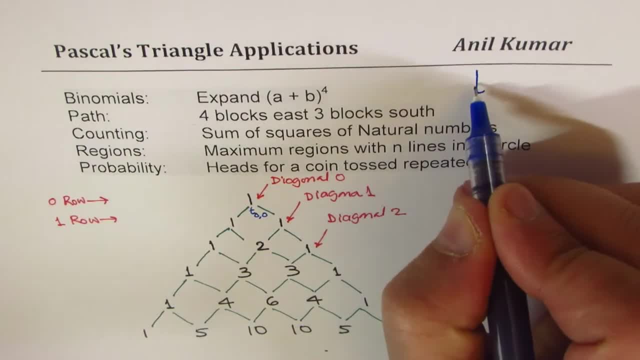 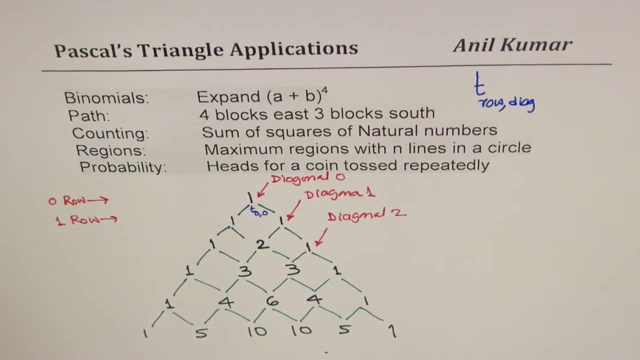 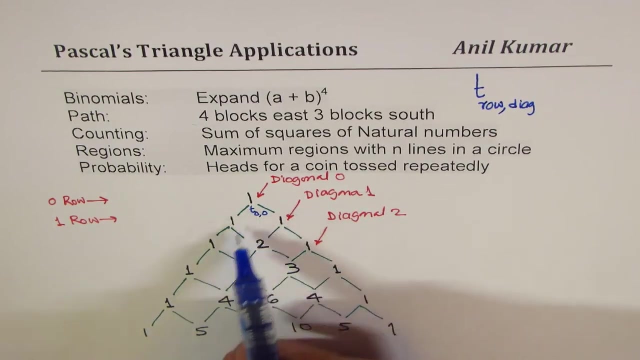 row and column, is it okay? so in general we'll write t for term and then we'll write row number, comma, diagonal. okay, so that is how each position is going to be identified. so this becomes the. so all these are t zeros, do you understand? all these are t zeros. so this term here will be for. 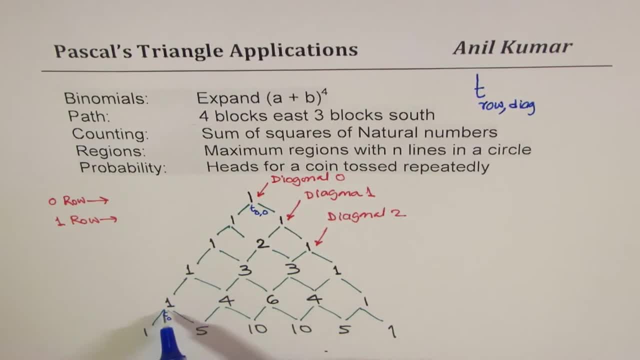 example t zero and the diagonal number is also- i'm i'm sorry- row number is four for it. so let me write four and zero, right. diagonal is zero, row number is four. so let's get back to this. row number three, right. so we'll write t three here and diagonal is zero, comma zero. that is how you're. 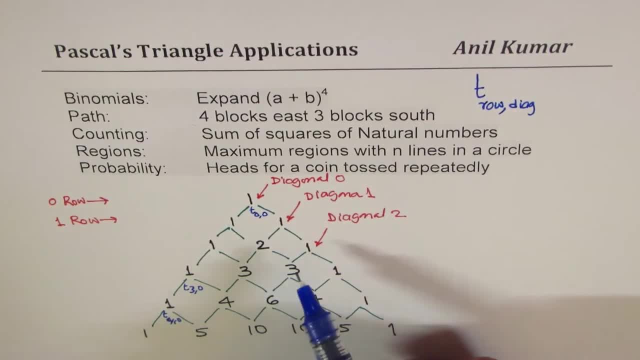 going to get the term numbers, because we're going to get the term numbers, so we're going to get the correct. so, for example, position number six, position of six, here is in the row four right, so this will be t, t four. four is for row number and as far as diagonal is concerned, it is diagonal. 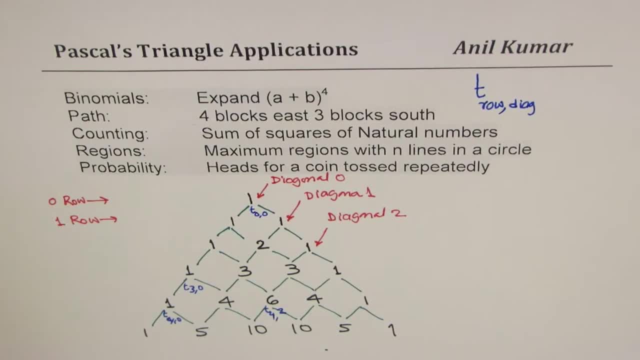 two. okay, so that is how we are going to treat it now. this is a very interesting pattern. we'll only answer the questions mentioned here, but let me tell you how you're going to get the term numbers right. so let me tell you how useful this is. i'll provide you with links which will give you a lot. 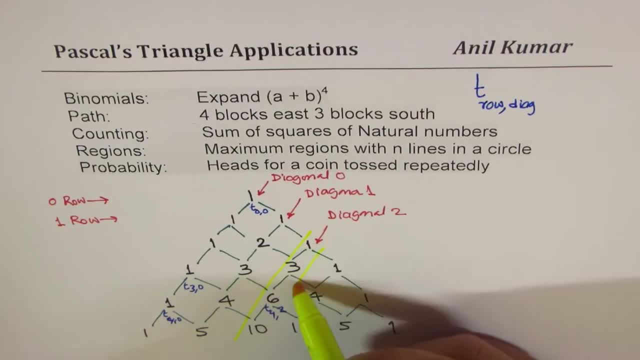 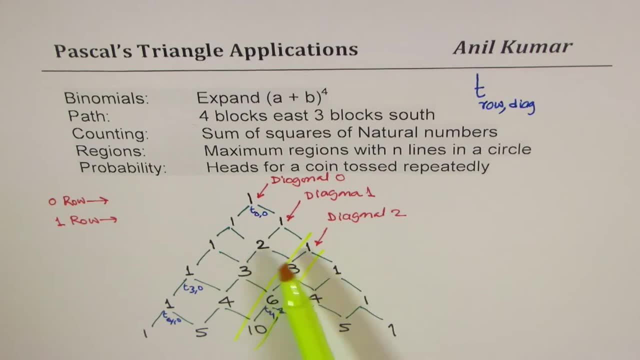 of information about this. these numbers right here: one, three, six, ten, they are called the triple numbers, right, and they also give you some of natural numbers. if you add just one number, you get one. if you add one plus two, you get three. one plus two plus three, six. one plus two plus three. 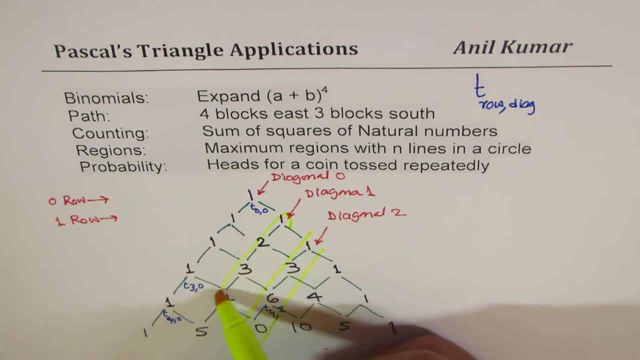 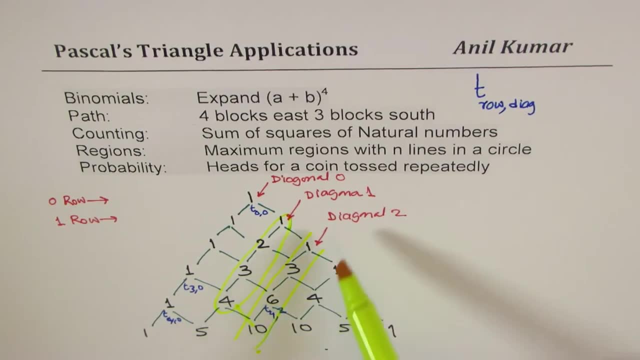 plus four is ten. right, so which is? you could think like this: one plus two plus three plus four is ten. next number will be plus five, fifteen. so these are the, uh, the triple numbers which we get, and similarly, uh, you know, if you get to the next diagonal diagonal four, we'll see how, what this. 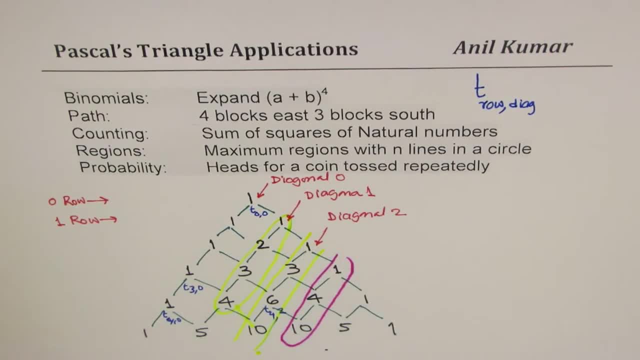 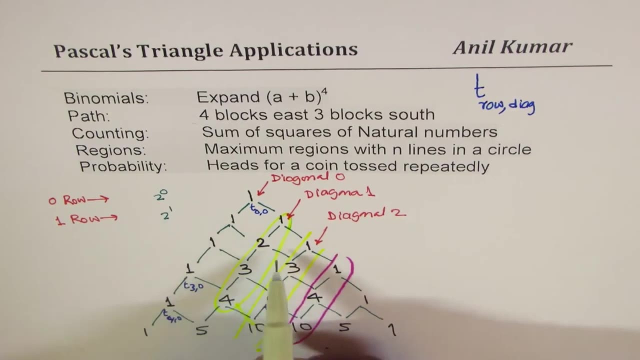 represents? this represents the combinations of tetrahedrals, right, so like this, it has many applications. if you sum these numbers like, this is one, right, so one is like two to the power of zero. this is two, which is two to the power of one, and the sum here, 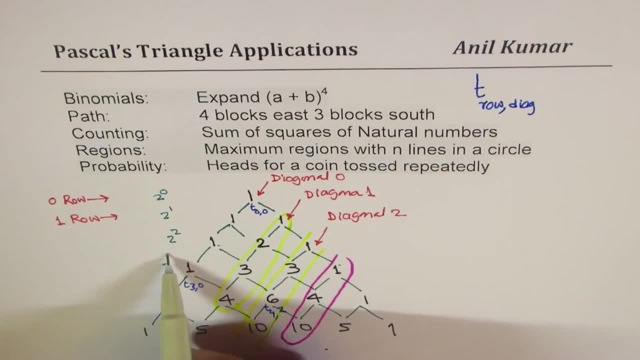 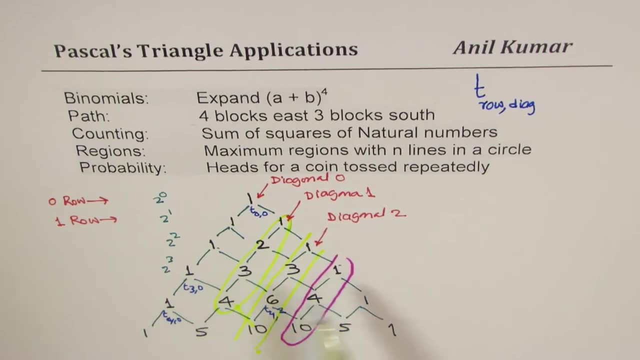 will be two to the power of two. sum here will be two to the power of three. right one plus three is four. four plus four is eight. you'll also see symmetry here. from left to right, as you move, all the numbers are symmetrical, correct? if you're looking into rows with prime numbers. 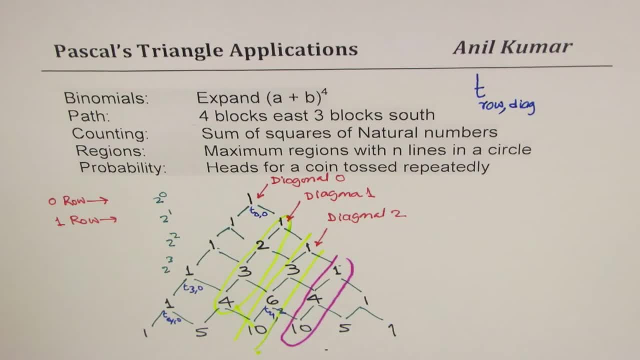 they are multiples of that prime number. so there are many properties which we'll discuss in other videos, but i hope you get good picture of this. let's begin by answering the first question. so let me now discuss binomial expansion with the help of this particular application. so we're talking about 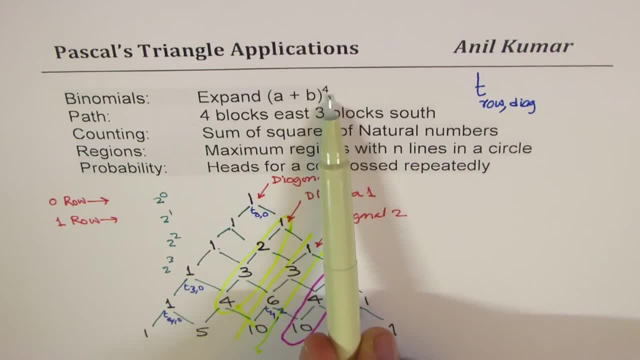 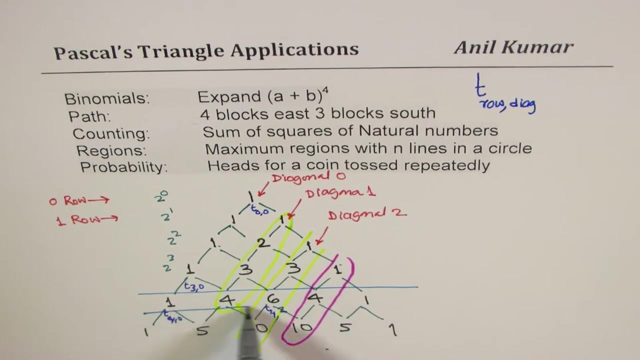 now expanding a plus b to the power of four. that means we look into the fourth row. now which one is the fourth row for us? we are calling row number zero, row number one, two, three, four, so that becomes our fourth row, do you see that? so in fourth row you see the numbers one, four, six, four, one. 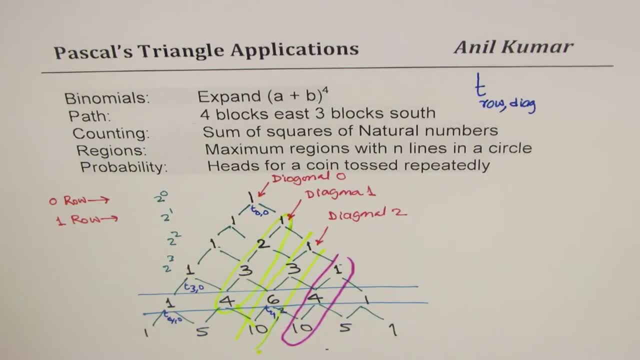 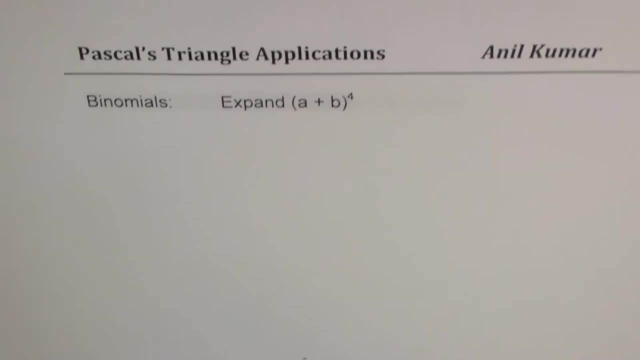 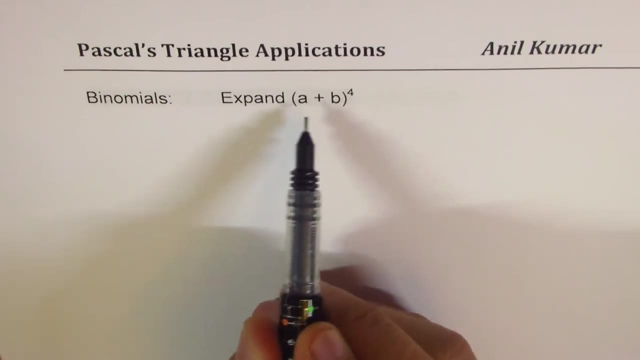 which will be applied in the expansion of a plus b to the power of four. so let's take this now as a fresh page. okay, now let us see how to expand a plus b to the power of four. now, these are binomials. if you have two terms, we call this binomial. the expansion of this can be: 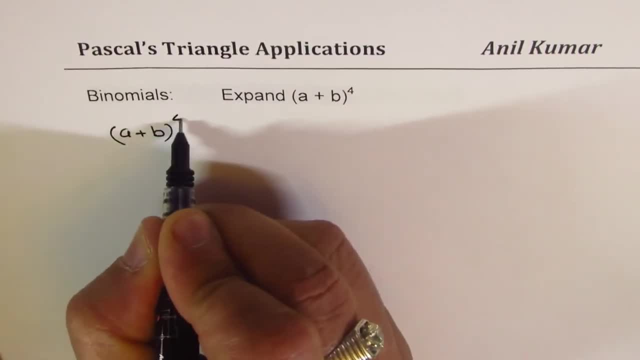 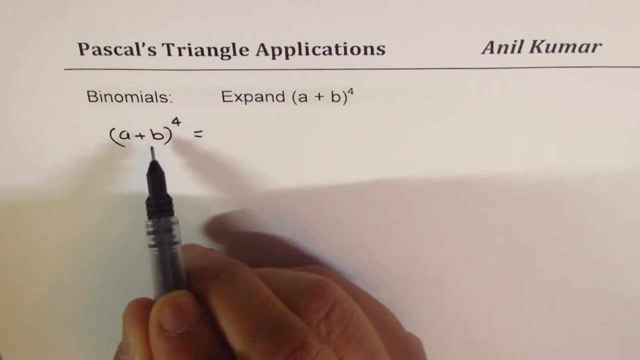 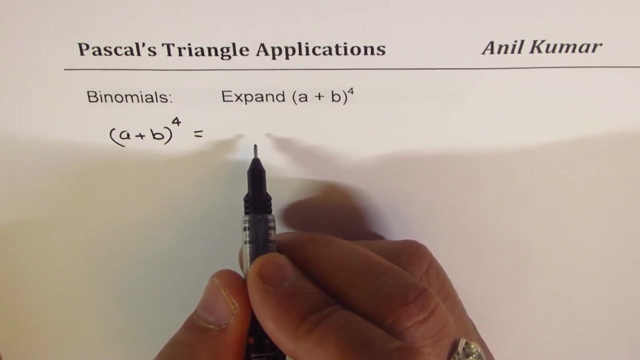 done with the help of pascal's triangle. i'll show you how well. whenever you expand with binomials, with such power, the power of combined power of both the elements will always be four. right, so what? we are going to get here one. so when you expand a plus b to the power of four, we'll 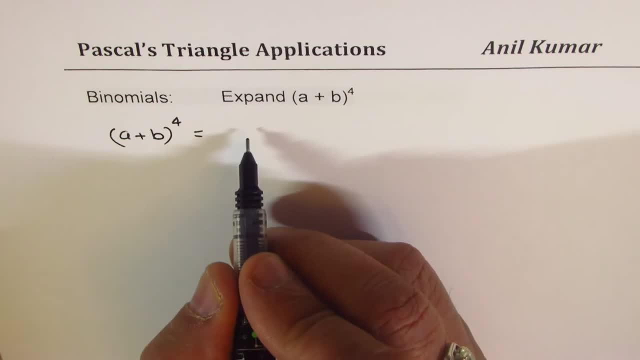 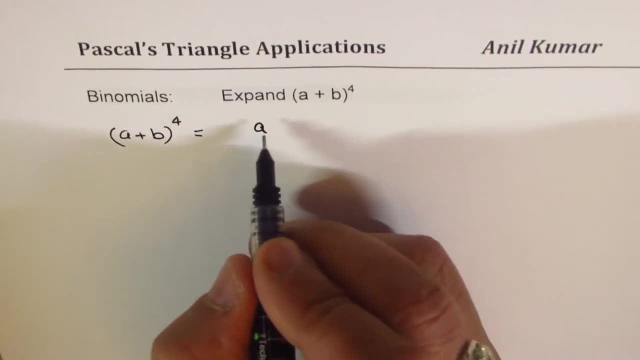 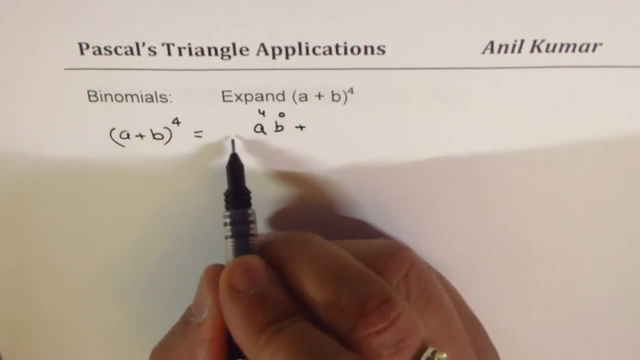 actually get five terms. each and every term will have combined power of a and b as four and be in a particular order. so you will notice that a and b both are there. power of one increases and the other decreases. so let's put power of four on a and zero and b and we'll continue this kind of a series, leaving some blank. 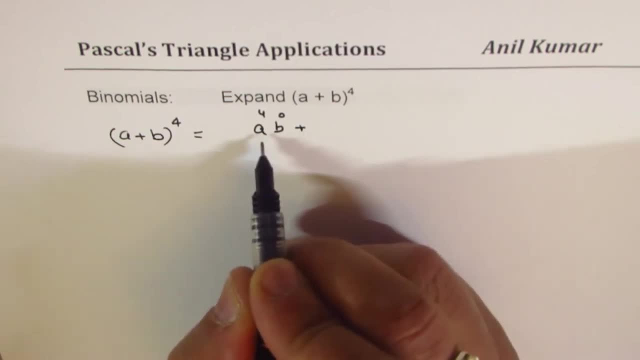 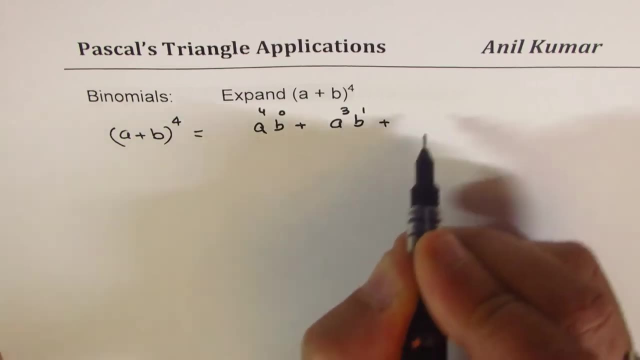 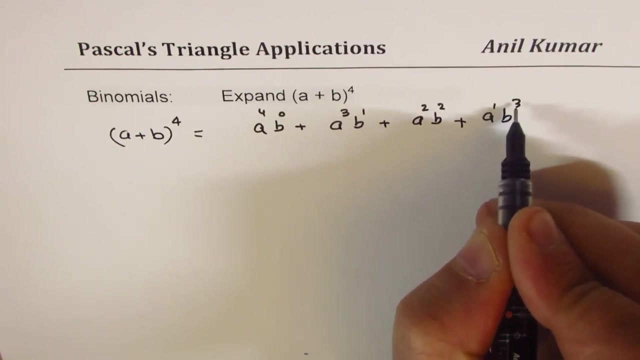 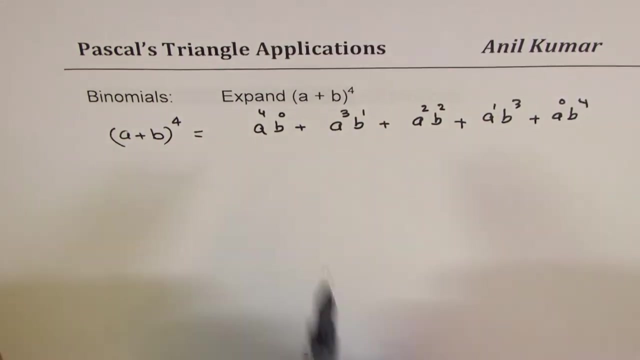 here we'll see how to fill those blanks. we'll call them coefficients of these terms. so we could get a cube: b to the power of one plus a square b. square plus a to the power of one, b, three. so three plus one is four, and now we have a to the power of zero, b to the power of four. so we'll 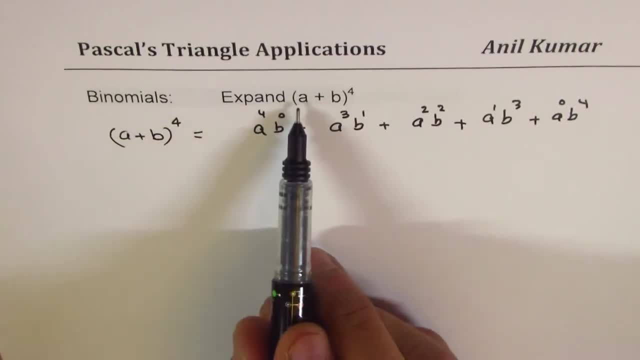 get actually five terms whenever we expand a binomial expression with four. so if it is n, you'll get n plus one terms. now how do i get the coefficient of these terms? that is where the pascal's triangle comes in, right. so we'll again build up the pascal's. 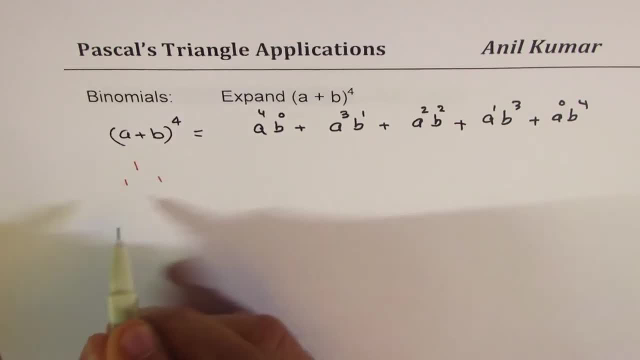 triangle. it is easy to make start with one and it'll give you practice. on the sides it is always one right, so on the sides it is always one. in the center you have to add the two above, so one plus one is two. so that is the second row. we have to go up to the fourth row, so this is the third row now. 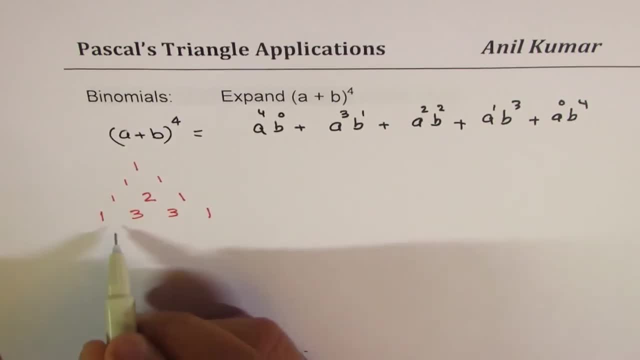 adding one and two, we get three. two plus one is also three. and now the fourth row, once on the side. one plus three is four. three plus three is six. three plus one is four. so that is your fourth row. now. these numbers here are the binomial coefficients, right? so these are the 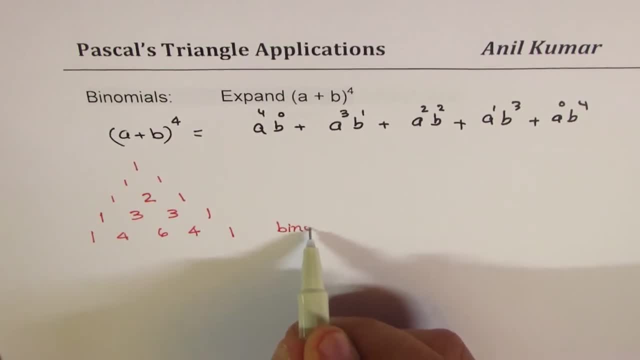 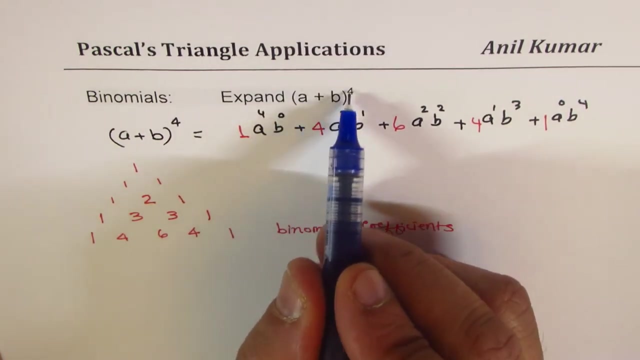 binomial coefficients. let me use the term binomial coefficient, so binomial coefficient, so i'll put these binomial coefficients here. so we get one here, four, six, four and one. so they are directly placed. and that is how you get the expansion of this binomial a plus b to the power. 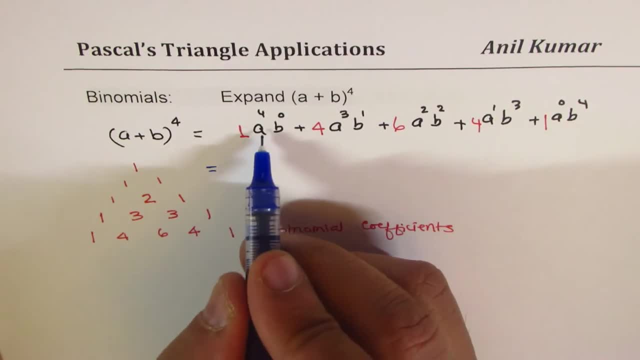 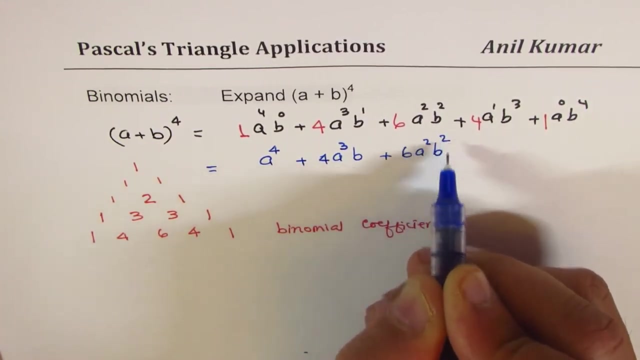 of four. let me rewrite this properly: that is one, no need to write. so we'll write a to the power of four. anything to the power of zero is one, right. so it is just a to the power of four plus four. a cube plus six. a square b. square plus four. a b cube plus b to the power of four, correct. 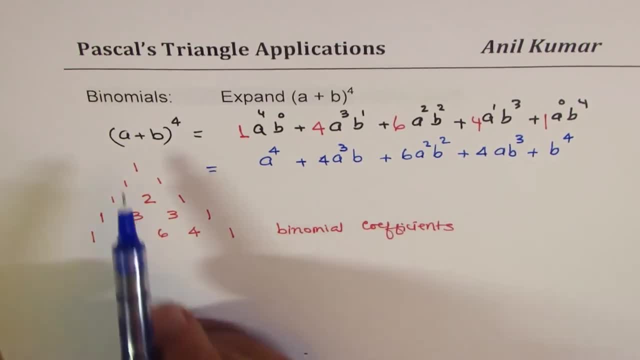 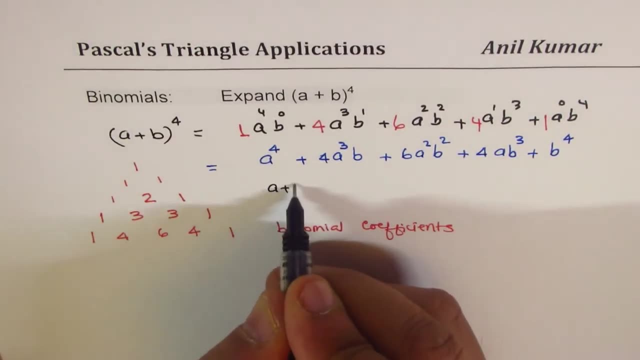 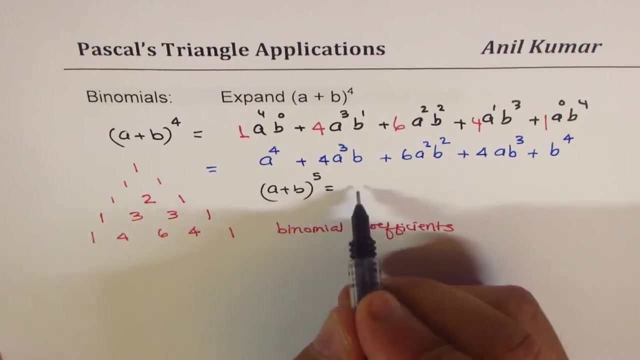 so that becomes the expansion of a plus b to the power of four. now, as an exercise, you could try out what is a plus b to the power of five. right, just expand this one more layer. you'll get six terms here. so you're looking for six terms. 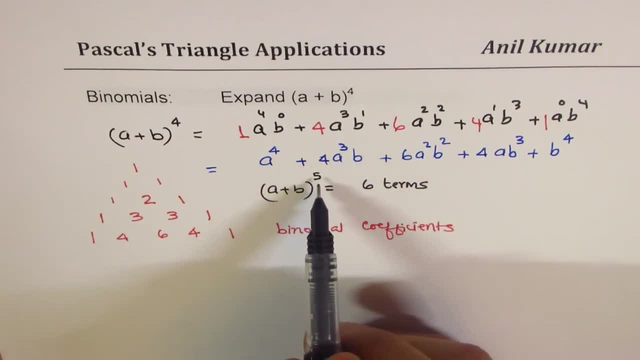 here. so you're looking for six terms and when you add the powers, it should always be five, correct? and the coefficients will come from here. coefficients will come from here when you add this, right, those are the coefficients which you have to build on. now. that was easy. you could do that. but if i say, write down what should be a plus b to the power of 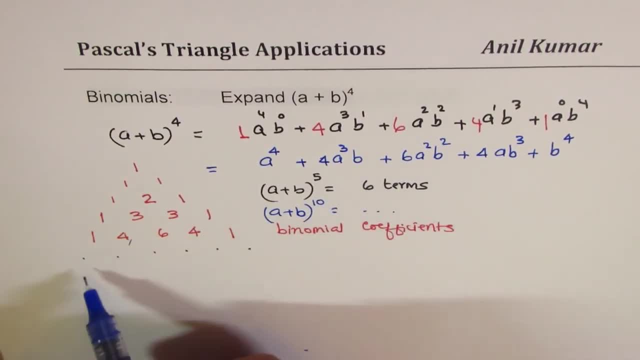 let's say 10, right now. this is very difficult, since how long can you make your pascal's triangle? so we'll actually introduce you to binomial coefficients. we normally write them as NCR, right? so instead of each term here is referred to as TNR, right so? 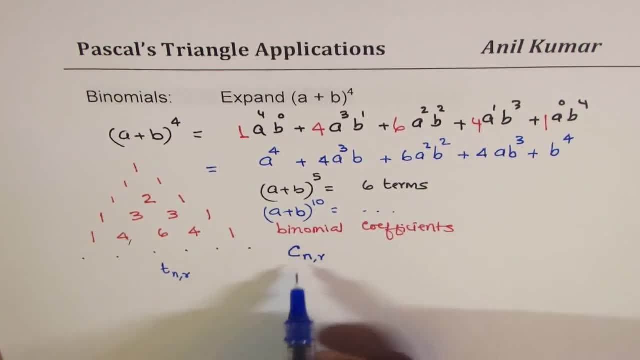 we write this as CNR and this helps you to do the calculation easily. in terms of N and R. it could be written as: N factorial divided by N minus R. factorial times, R factorial. is it okay here? N and R is definitely the row number. it will help in here. we have switched. you know, it is N is the. 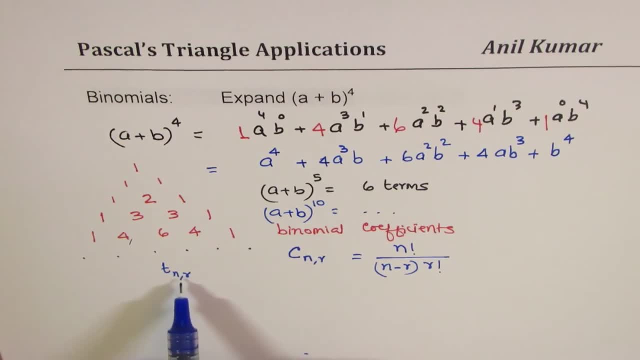 row and R is the diagonal. remember that correct? so that is kind of a switch here, but Either way, n has to be greater than r. That is very important, right? So this combination basically gives you that if there are n items and r to be selected, 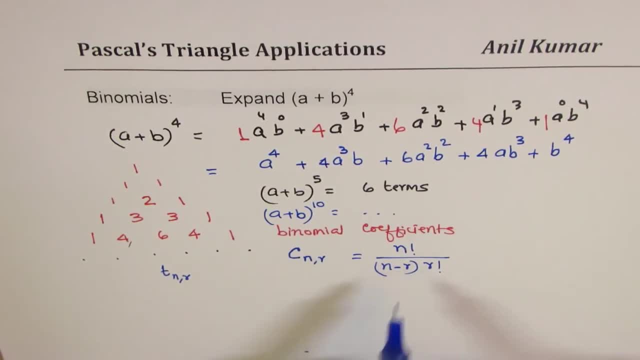 how many combinations do you get? So it answers directly that question. So it is kind of like the same thing. okay, What is n factorial? Let me teach you that also. n factorial is kind of. let's take an example. 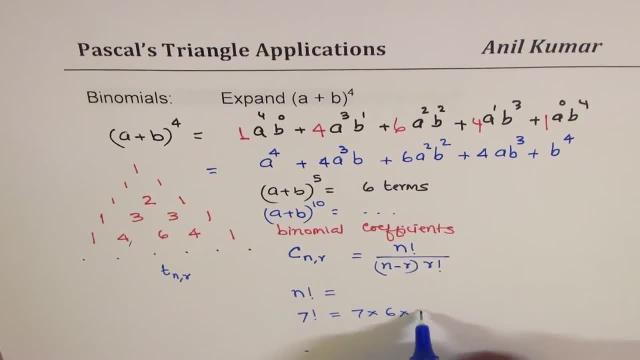 7 factorial will be 7 times 6 times, 5 times, 4 times, 3 times 2 times 1.. n factorial will be n times n minus 1 times n minus 2 times, so on till you can say at the end you will get 2 times 1, correct. 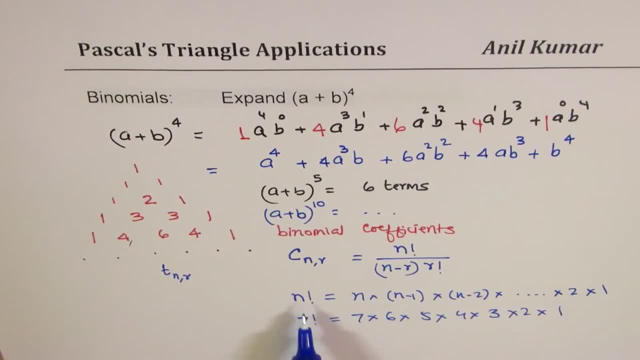 So that is how you are going to get n factorial And this helps you to calculate these numbers. To give you an example here: okay, let's take an example. Let's say we want to figure out this number, which is basically t, fourth row, 0,, 1,, 2, right. 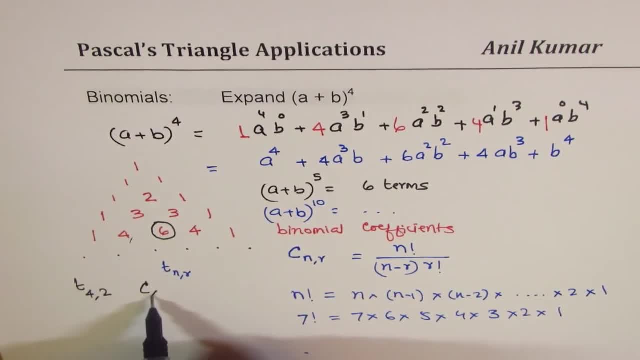 0, 1, 2.. So we will write this as c, 4, 2, and that is 4 factorial divided by 4 minus 2 factorial times 2: factorial correct: 4 factorial is 4 times 3 times 2 times 1, 4 minus 2 is 2, right. 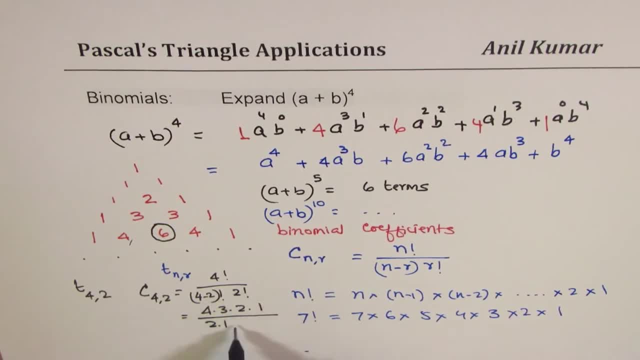 So we get 2 factorial, which is 2 times 1.. This is also 2 factorial, which is 2 times 1, correct? So if you simplify, what do you get? This 2 cancels with that. this 2 cancels with this 2 times 3 is 6.. 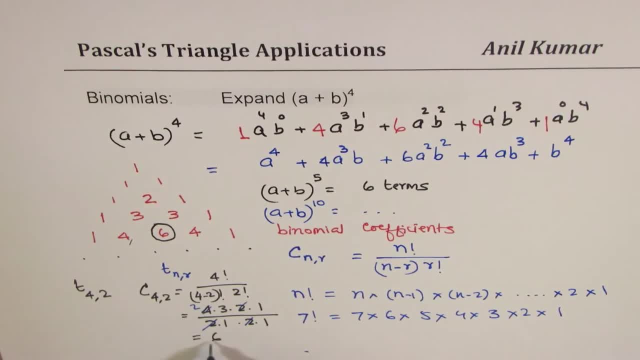 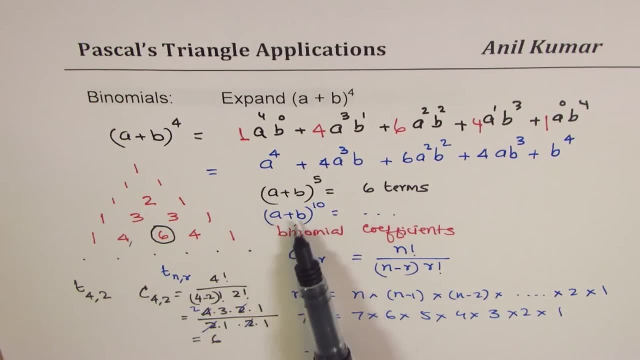 So you do get 6 here also, right, You get the same number, 6.. Likewise, you can calculate all numbers. So now your question is: you have to now write expansion of a plus b to the power of 10 using this formula, right? 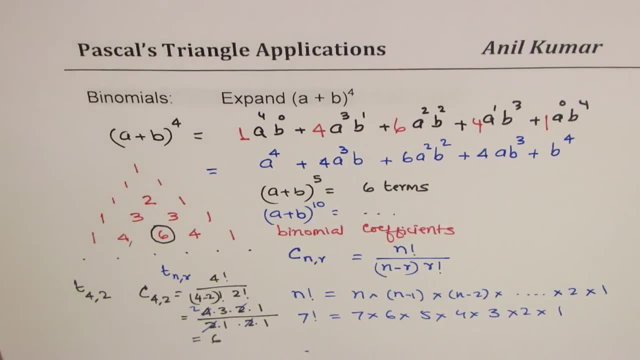 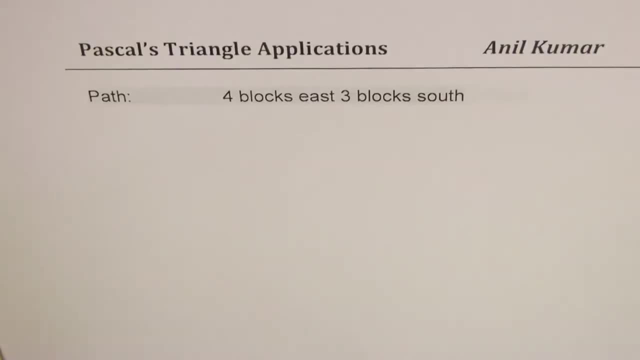 So I hope that becomes interesting. So let's move on. So you can see how Pascal's triangle and now I've introduced binomial coefficients are also related. Let's take up the next thing, which is counting the number of parts. 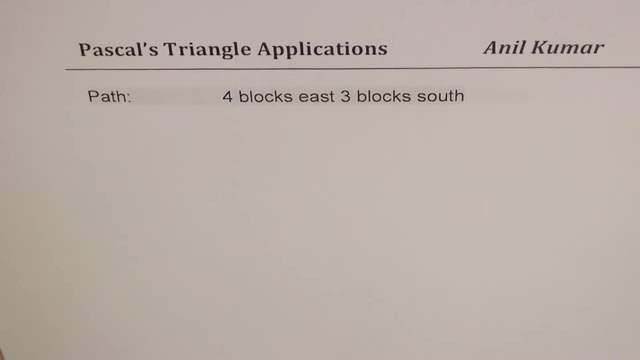 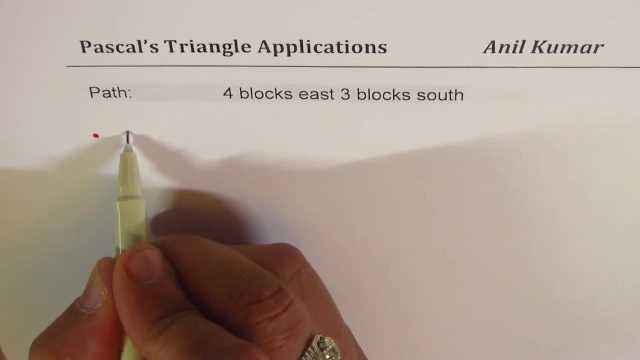 This is a huge application of Pascal Pascal's triangle. let us say- here is the example: We have to go 4 blocks east and 3 blocks south. That means, if you're in this location, 4 blocks east. so there's only one way. let's. 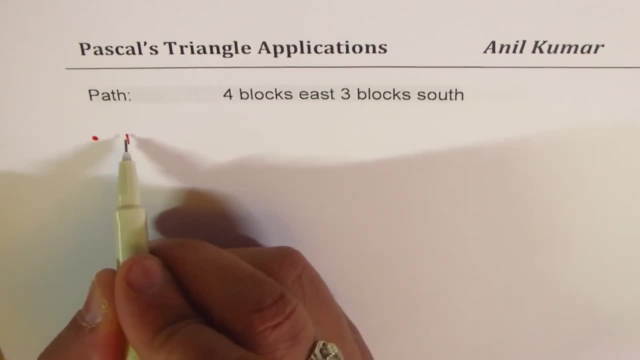 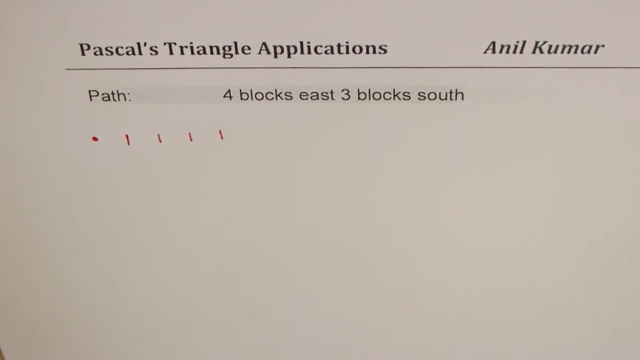 go 4 blocks east. East is this direction for me: 1,, 2,, 3,, 4, so you reach that point right, 4 blocks east, and you're supposed to go 3 blocks south. So let's go 1,, 2,, 3, 4.. 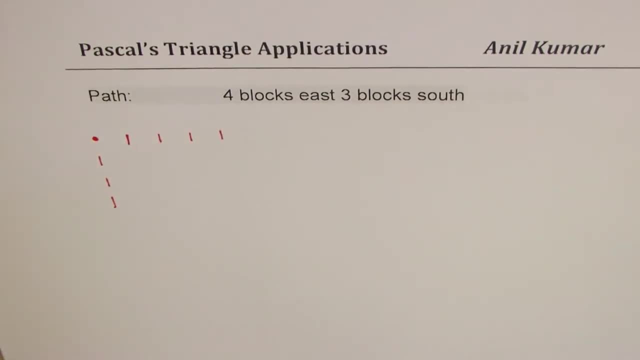 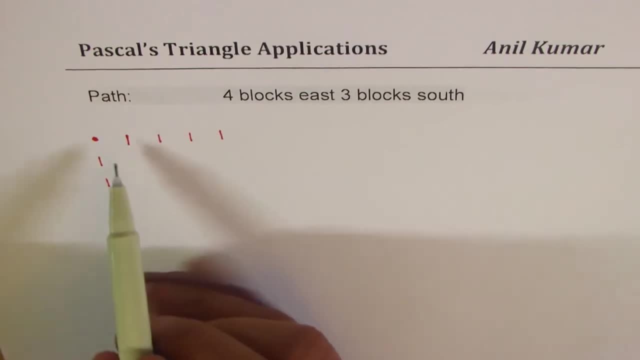 So what we're trying to see here. if you move in the east direction alone, there is only one way you can go. So those ones represent one way you can go. If you're moving only south right, So if you're moving only south, there is only one way you can go. 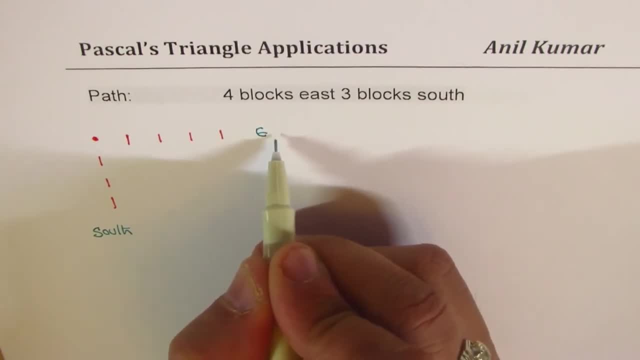 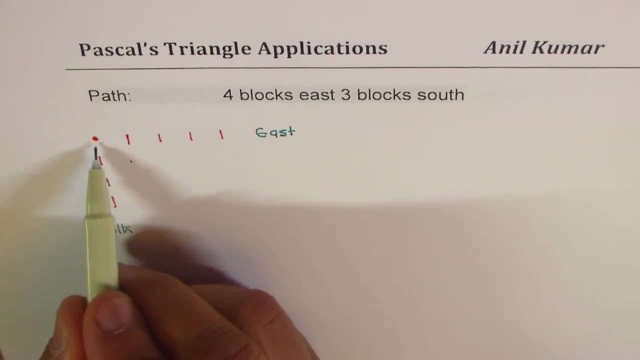 So these ones are representing, if you only move in one direction, correct? Now look at this, this position- you can reach this position from both the sides, so you can add them and then know how much should come here, right? so 1 plus 1 is 2, so you get 2 here. similarly, here you'll go 2 plus. 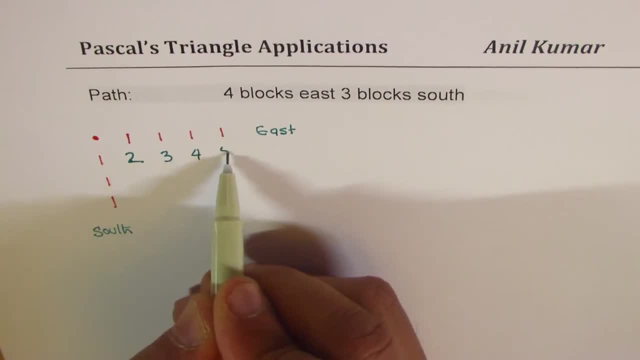 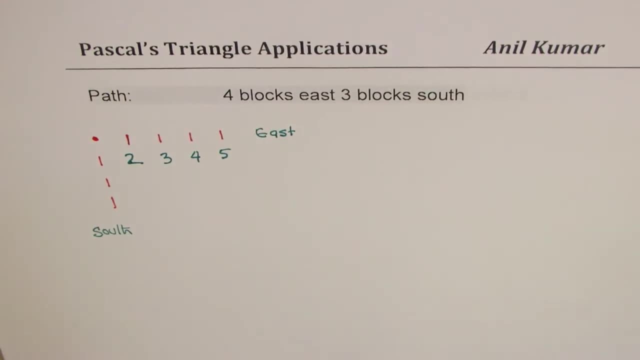 1 times, so we get the numbers 3, 4 and 5. does it make sense to you, correct now? next line, next line: here i could reach from this side. this is one way. from this side there are two ways. so 2 plus 1 is 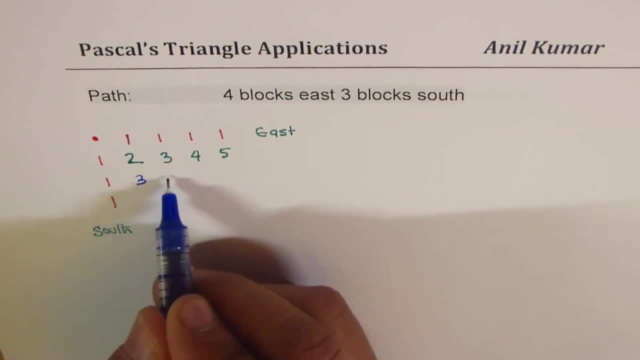 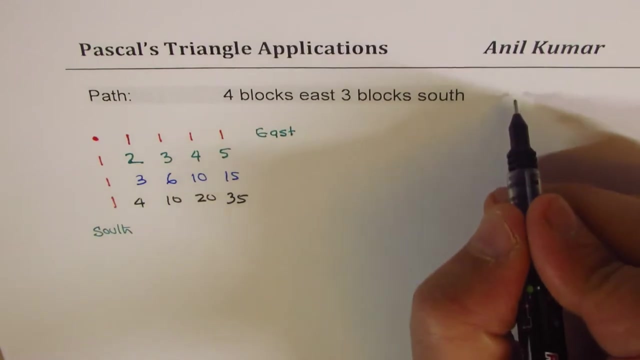 3, so we get 3, and similarly, 3 plus 3 is 6, 6 plus 4 is 10, 10 plus 5 is 15, so you can build on this. and here 3 plus 1 is 4, 4 plus 6 is 10, 10 plus 10 is 20, 20 plus 15 is 35, and so our answer is: 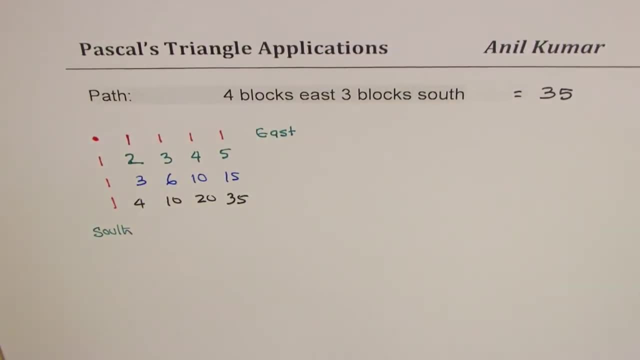 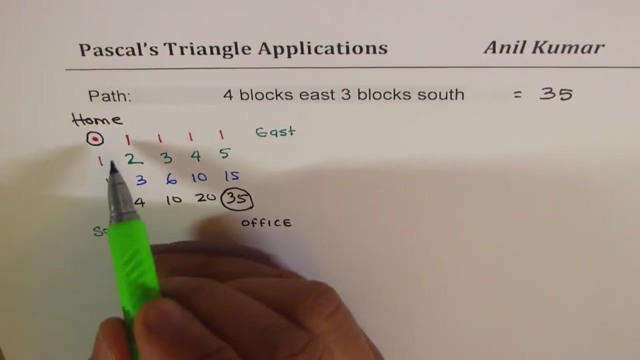 there are 35 ways in which you could go from one location- let's call it home- to the other location- let's call this as office, let's say, right, so let this be office, okay. so i mean you understand. different paths means we have all such combination we could go. 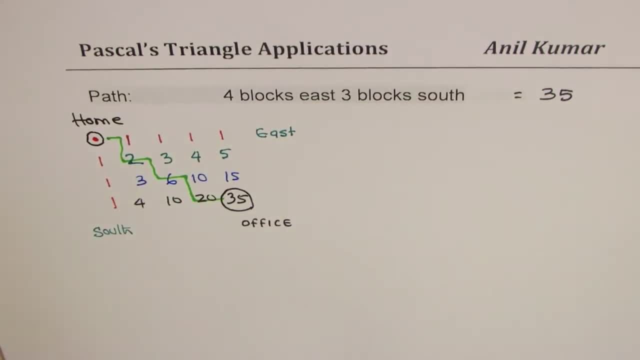 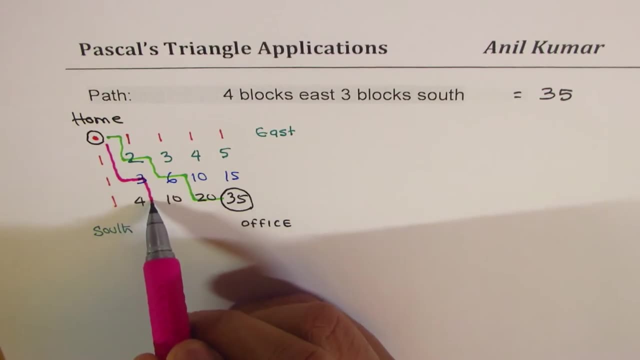 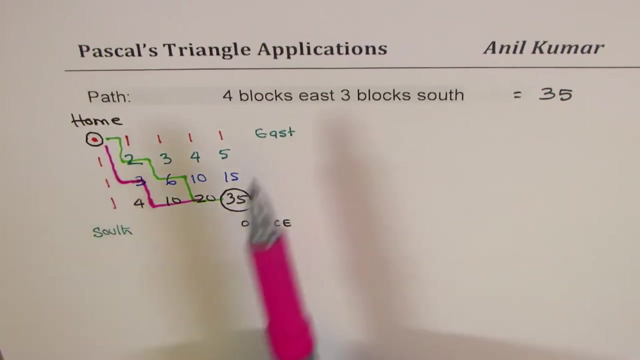 like this right, or you could take some other path if you wish. like wish to right. so you could go kind of come south first and then go like this. so there are 35 ways in which you can reach office from home. if you have to go four blocks east and three blocks south, perfect. so very easy way to use. 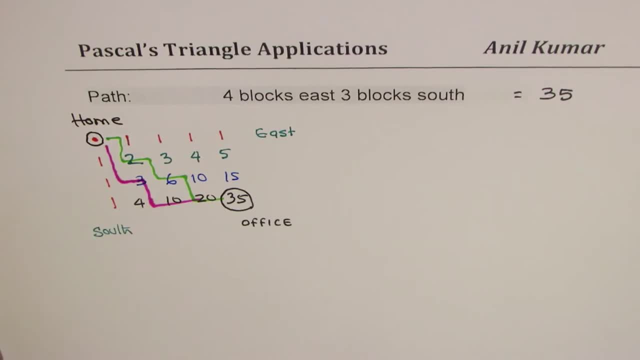 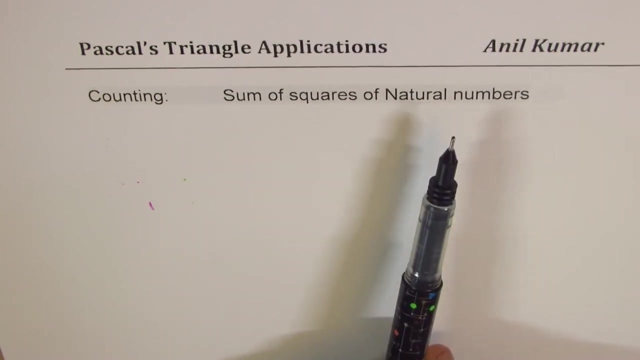 application. very easy way to apply pascal's triangle and answer such questions. now let's take up one question on counting principles. so the question here is: how do we find sum of squares of natural numbers? well, sum of squares of natural numbers. so let's make a table. let's make a table. 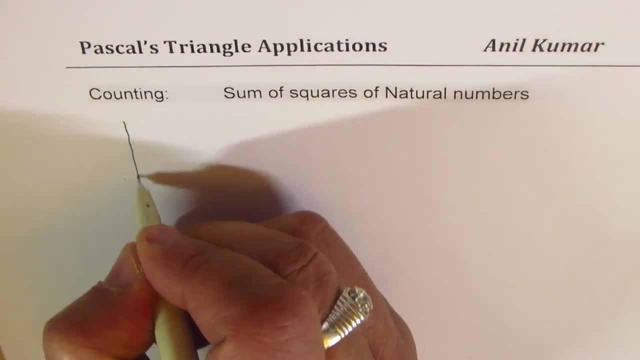 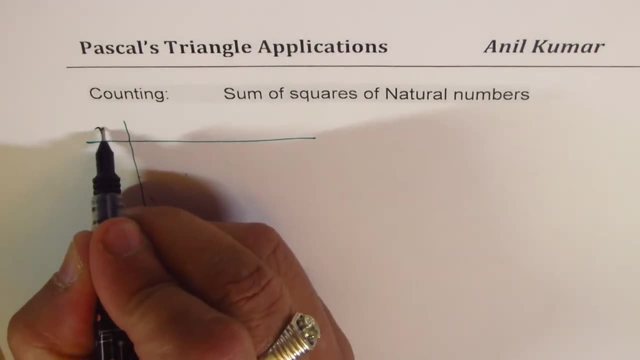 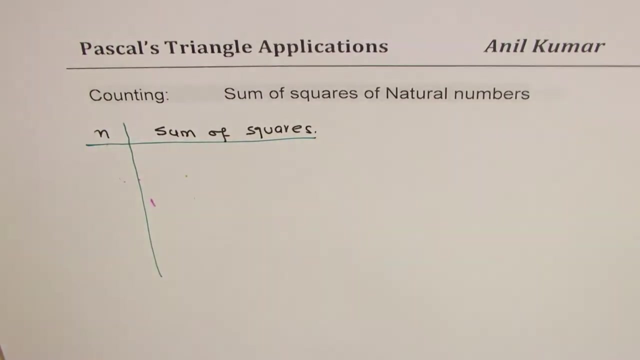 and then figure it out. so in this table i will take n, the numbers on one side, and we'll write some on the other side. so sum of squares. okay, let's take numbers one by one. so if i take one number it is one square, and you know what one. 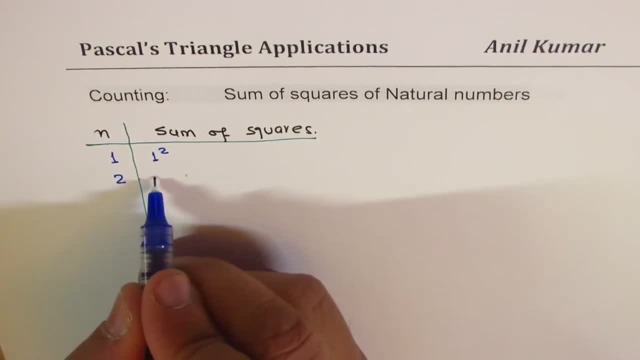 square is two. if i take two numbers, that means one square plus two square. it is sum of natures, sum of squares, of natural numbers, right? so if you take three natural numbers, so that means one square plus two square plus three square. that's what i mean, right? if i take four, it 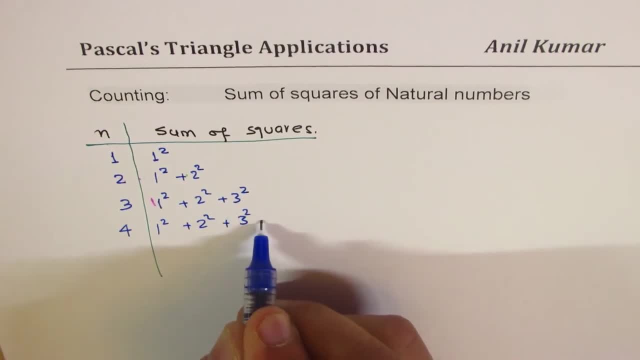 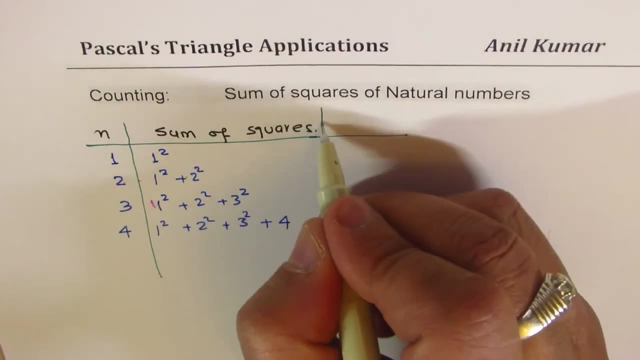 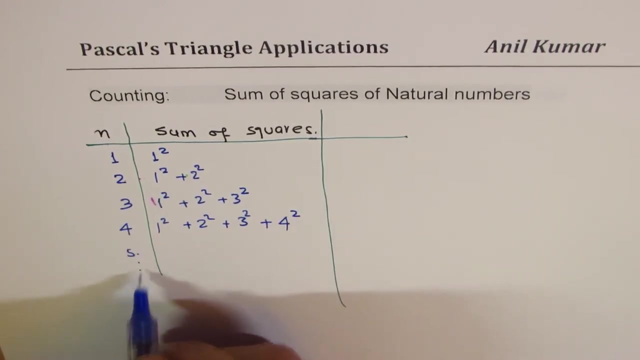 means one square plus two square plus three square plus four square, and so on. right, so let's see what their squares is. okay, uh, let me write square here and, like, the series can go on and on. perfect, now what is this square? so we might have to use the calculator. so let me look for a calculator. 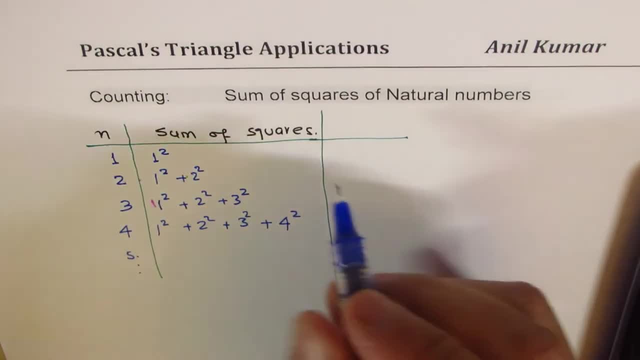 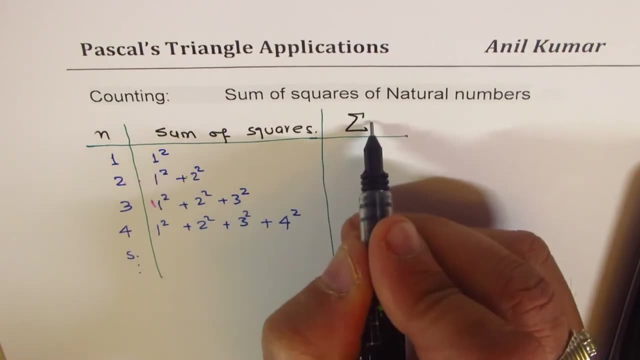 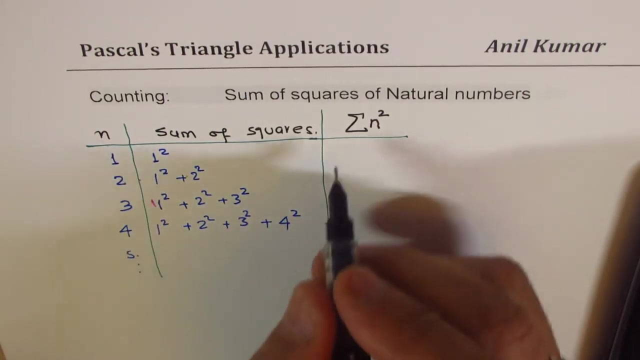 now, here we have one, and in this column we'll just write some of these squares, so let me use the notation Sigma. so we are doing sum of natural numbers, squares, right, that is what we're trying to do, okay, so one square is is one. one plus four is five. 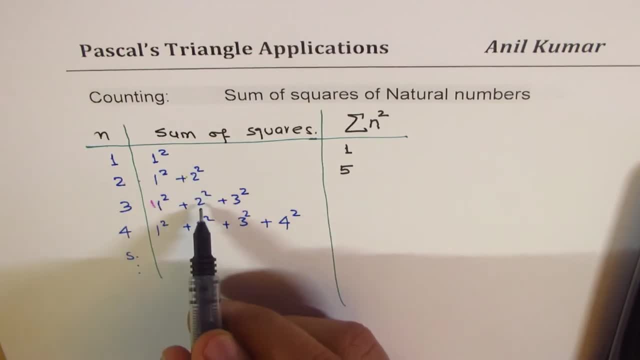 okay. one plus four, that is five. five plus nine is fourteen. okay, so we know up to here. and fourteen plus sixteen is thirty. okay, so that is how you can build on it, correct? so next will be five square. when you add this, it'll be like 55, right, when you add 25, and the series will move on and on. 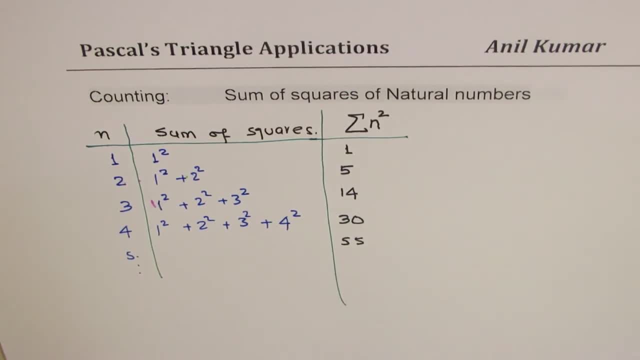 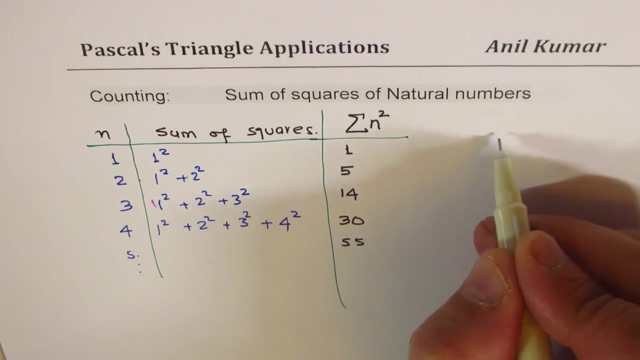 now, how do I get this using Pascal's triangle? fortunately we didn't use the calculator. okay, let's figure this out. so let me build the Pascal's triangle quickly and see where these numbers are, and then we'll try to figure it out. so let's start from here, for example, so we say one: 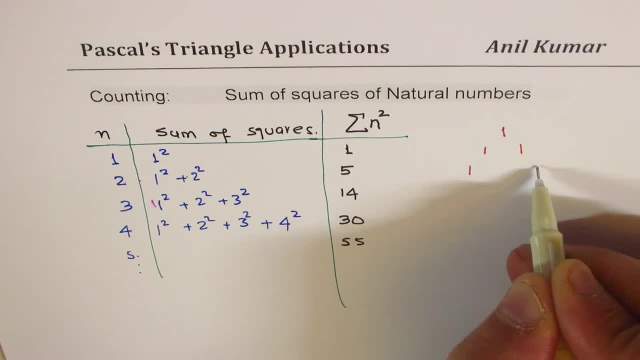 and then we go one, one, and then we go one, one, and combination here gives me two, one one. one plus two is three, two plus one is also three, and we have one, one on the side, three plus one, four, three plus three, six, three plus one, four, and we did till: 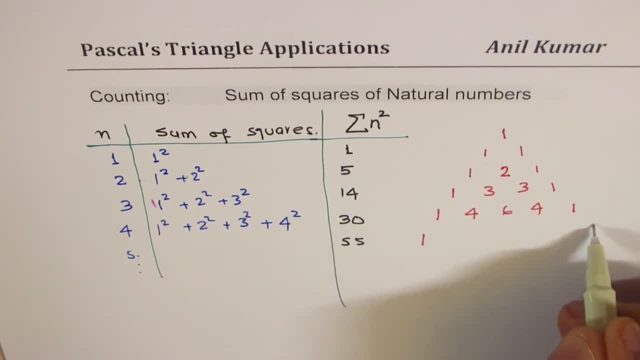 okay, and then we go again on the side and the side, and this: 4 plus 1 is 5, 10, 10 and 5. and let's go one more step here: 5 plus 1 is 6, and this is 15, this is 20. 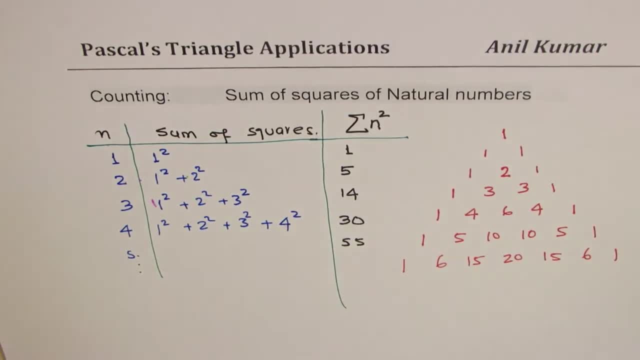 there is symmetry, as you can see, right, so like this, or we can go on. I'm looking for numbers like 1 plus 5. okay, we may have to go one more row. let's go one more row. so we have 7 here. 6, so you'll find this is prime number. 7, right, all? 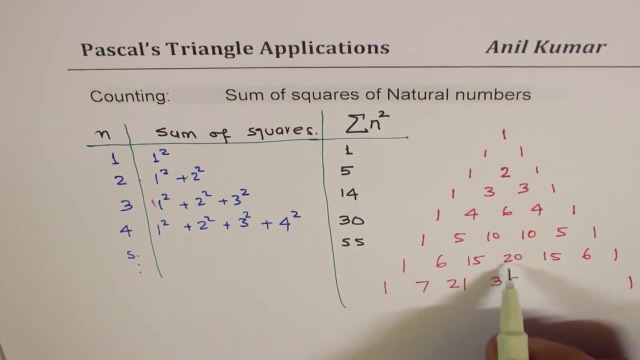 numbers will be multiples of 7, 35, and this is also 35, this is 21 and like this. now can you figure out how we can make this sum? how do you get 5, how do you get 14, and how do you get 30 and 55? so at times you may have to look very 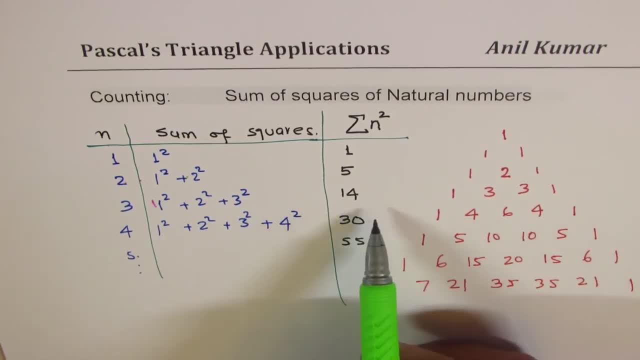 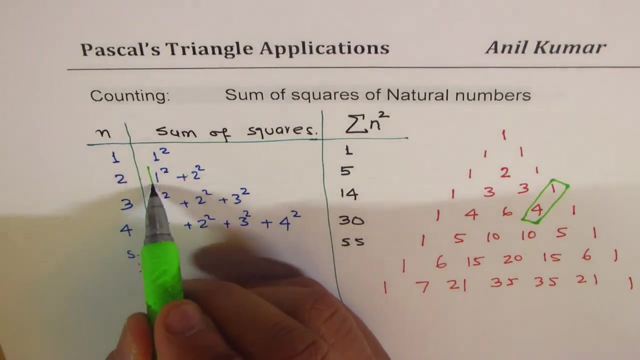 carefully for the numbers. so we are saying that sum of squares of first number is 1 and then second number is 5. so to get 5, one way is that we could add these two numbers, and when you add these two numbers you get 5. okay, so we got one. 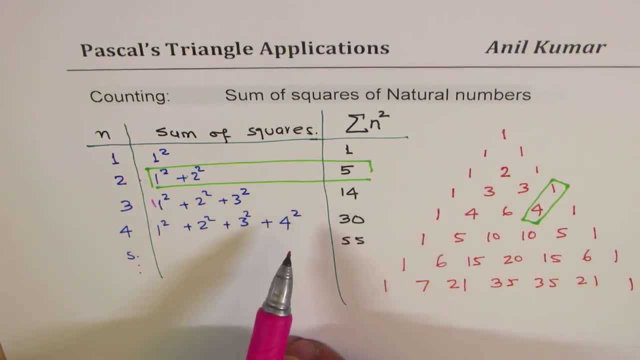 combination like this: now, how do I get 14? okay, to get 14, let me add these two numbers now. so so, these two numbers added, we get 14, right? so so, okay, we added, I mean this series. okay, then, how do I get the next number, which is 30? well, 30 is 20 plus 10. 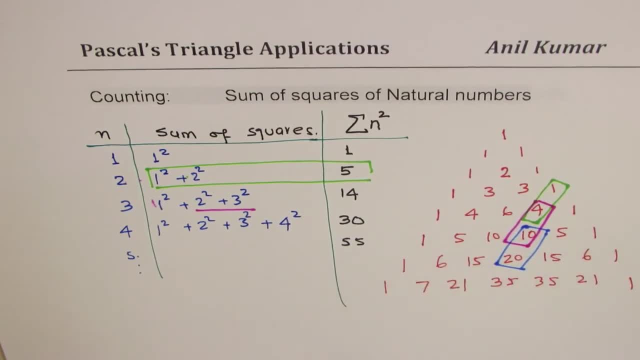 okay, so I add this: 20 plus 10, 30. that's good. so we got this number. also, how about the expected 55? well, at 20 and 35, does it make sense? so see, by this addition, we are able to generate sum of squares. that's the whole idea. we are able to generate sum of whole. 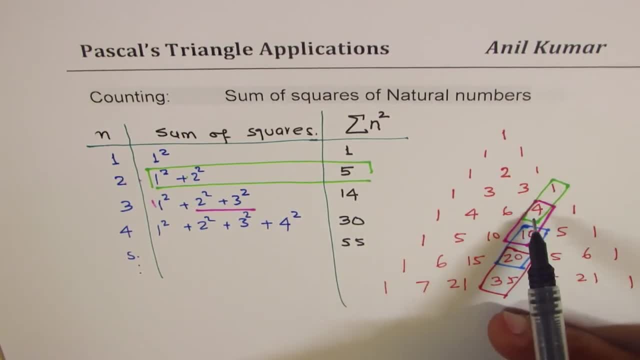 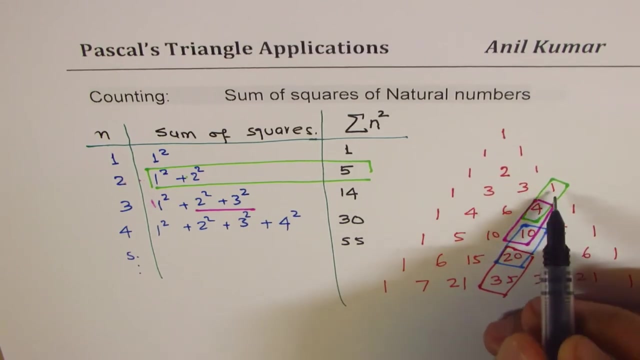 squares? now how could I write this in terms of Pascal's triangle? now, that is the trick. so what you have to do here is basically see the pattern and then make a formula out of it correctly. so the formula here is: we are adding these two terms. what is the term number? 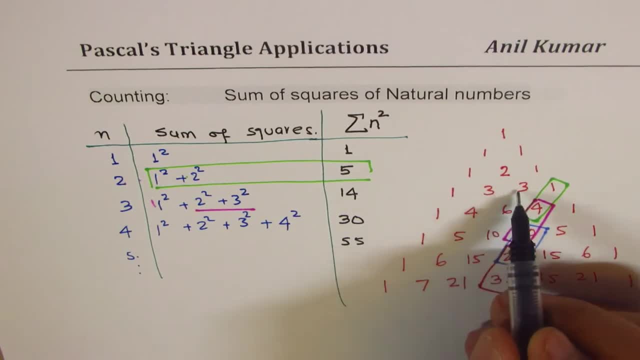 this is the third row, correct, and 0, 1, 2, 3, so I could write this as T 3, 3 plus. the other number is fourth row and 0, 1, 2, 3, so it is T 4- 3. do you see that, if you? 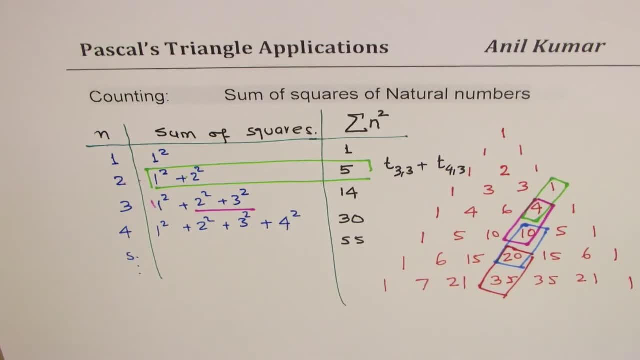 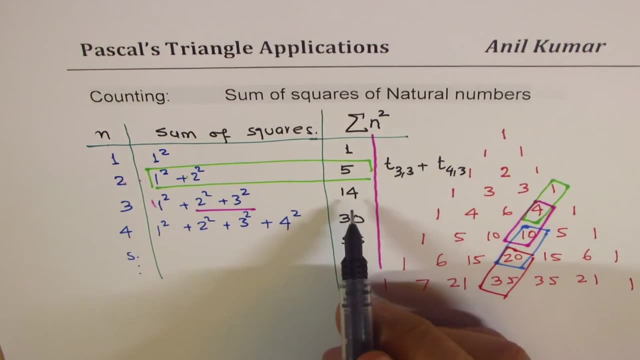 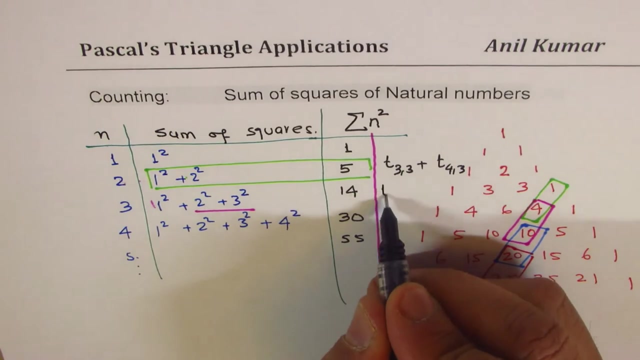 add this, you get your answer. does it make sense to you? so have a look. let's try out the next number, which is- or we should get 14, which is the sum of 4 and 10. and where is 4? 4 is in the fourth row, so T 4 and the position is 0. this is 0. 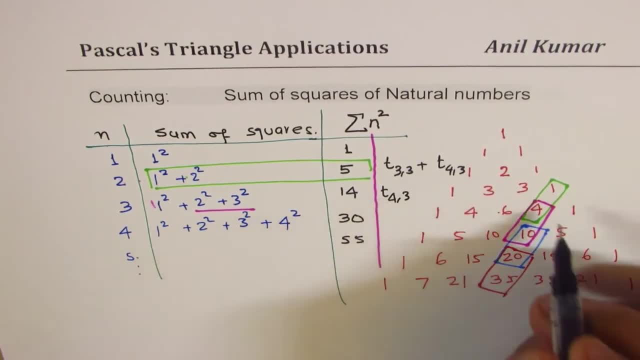 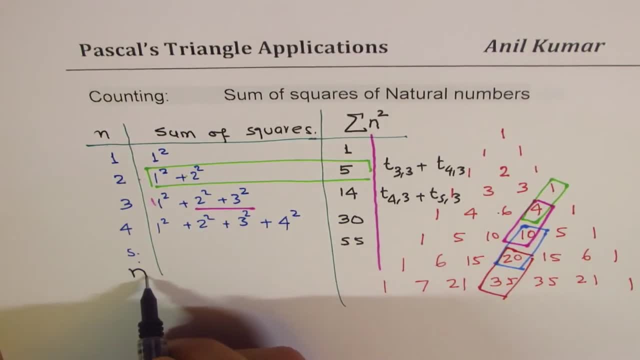 T 4 is in the fifth row. okay, so T 5: 3. so you see the pattern. so in T 4 is in the fifth row. okay, so T 5: 3. so you see the pattern. so in general, if I have n here, then what do I? 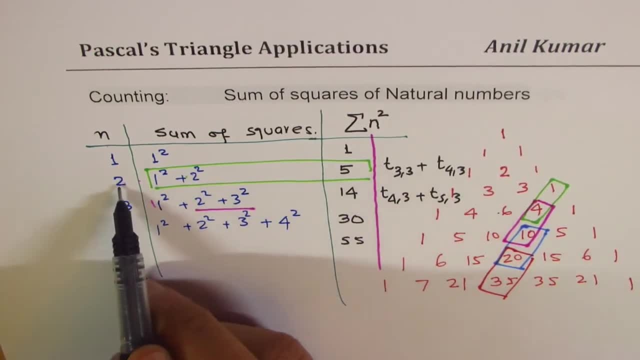 general. if I have n here, then what do I general? if I have n here, then what do I expect? now, these numbers 2 is 1 more than expect. now, these numbers 2 is 1 more than expect. now, these numbers 2 is 1 more than 3. right 4 is 1 more than 3, so I should. 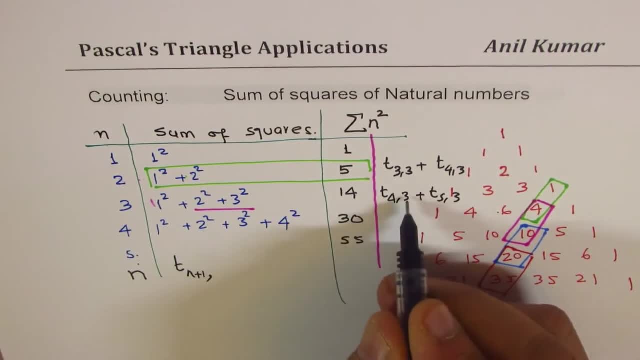 3 right. 4 is 1 more than 3, so I should 3 right. 4 is 1 more than 3, so I should get T n plus 1, but diagonals are 3 okay. get T n plus 1, but diagonals are 3 okay. 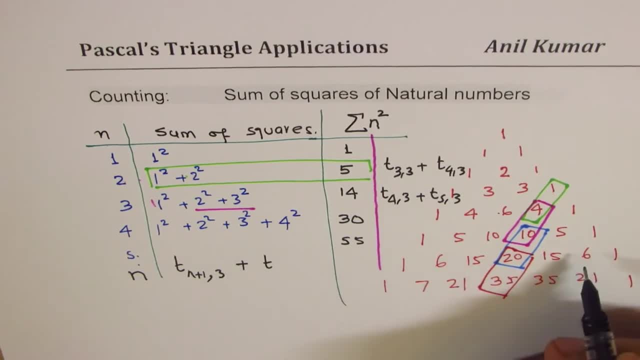 and the other term which you add to is the next row. so more than one, so n plus 2, third diagonal. so that becomes your formula to find the sum of squares of natural numbers, correct. so now what you can do is you can find sum of first, sum of squares of: 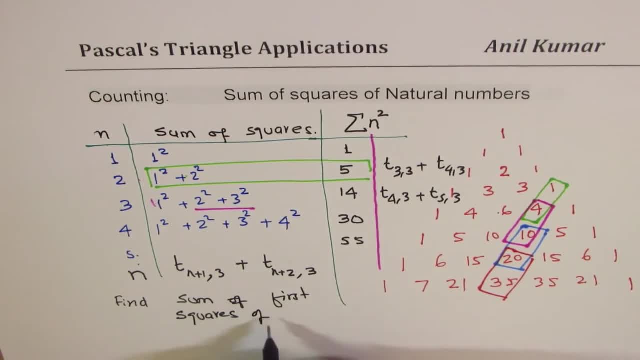 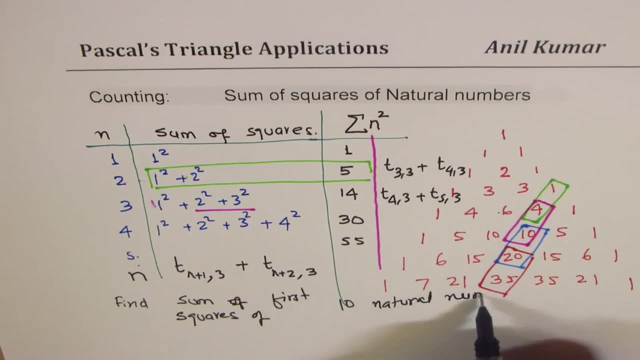 first 10 natural numbers. let this be your exercise, okay. so what i'm trying to say here is: if i write in short, i want you to write: what is the sum of natural number square? what is the sum of natural number square? what is the sum of natural number square? 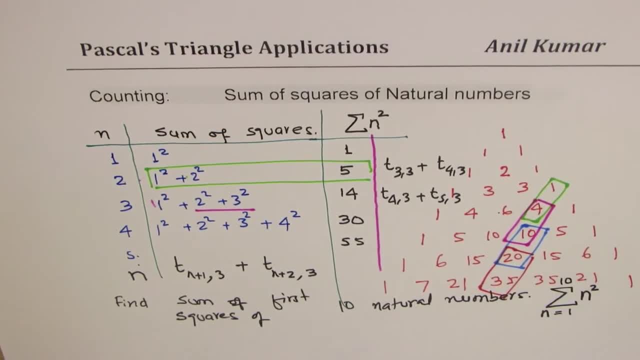 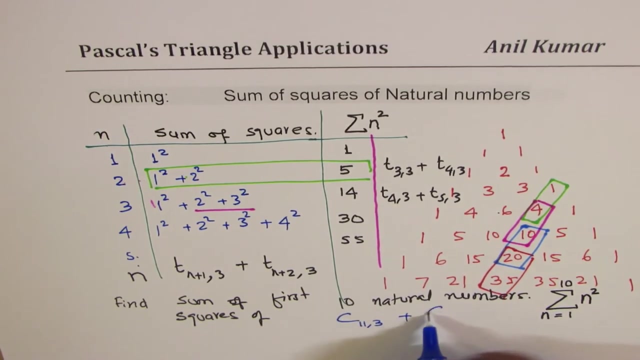 where n is changing from 1 to 10, correct? this is what you have to figure out now. either you build a triangle like this or you can use my combination formula, which is let in this term: right? so n is 10. so we get 11, c, 11, 3 plus c, 12, 3. that becomes the answer, right, so combination. 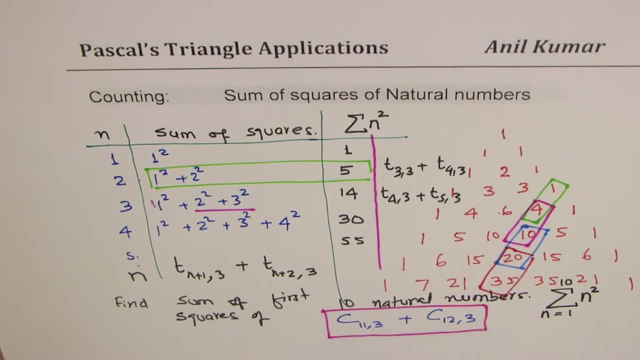 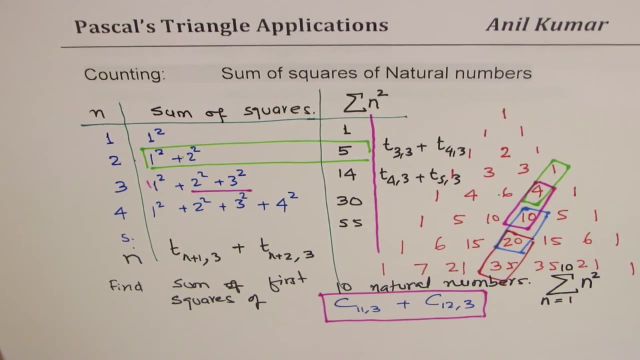 helped without making the triangle. you could do like this also, but it's not difficult to go up to 10. we are already at 7, perfect, so you could go right. so that is how we could do sum of squares of number. but i hope this formula is helpful right now let's move on and take regions which 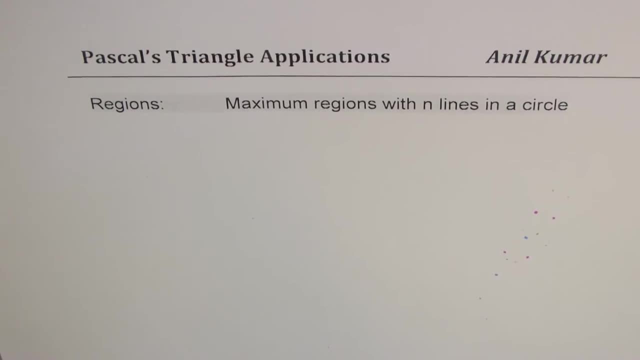 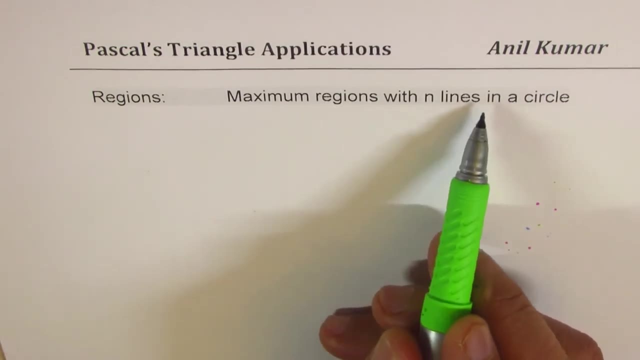 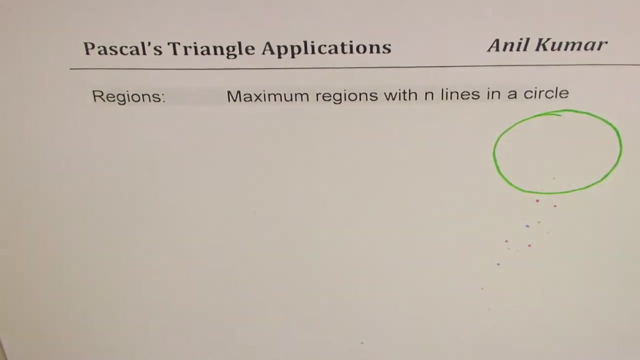 a circle can be divided into using lines. now the question here is: find the maximum regions with n lines, a circle can be divided, right? so basically look at it like this: let's say we have a circle here, right? so we have a circle. we'll make a table, as we did earlier, to 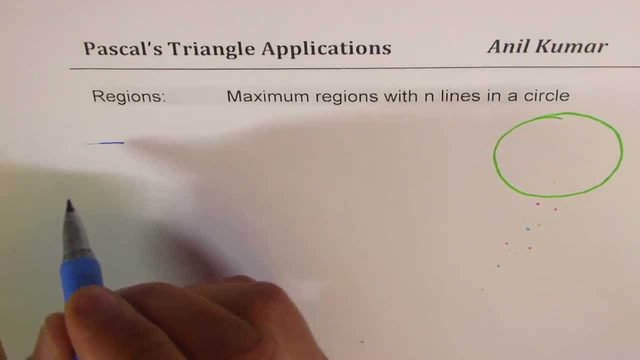 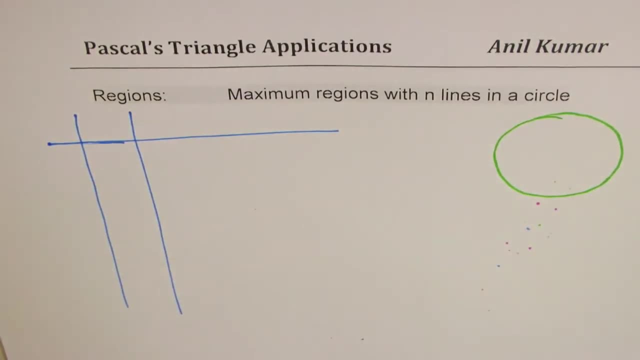 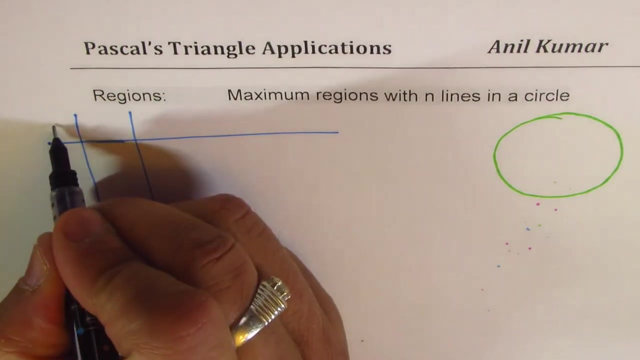 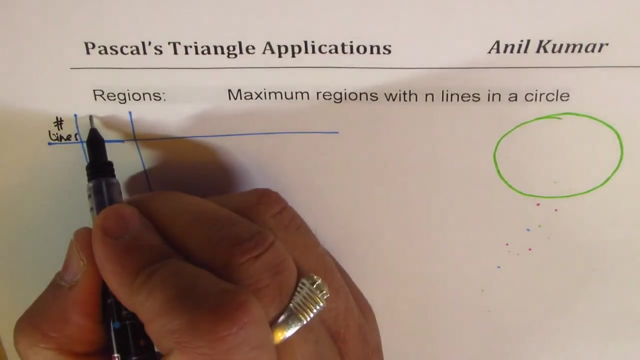 write down some values and then we'll try to figure out a pattern, correct. so so here is a table. okay, so we'll make the columns later. the idea here is that if we have n number of lines, let's say this is your number of lines, then how many regions do you get? so we want to find number of regions. 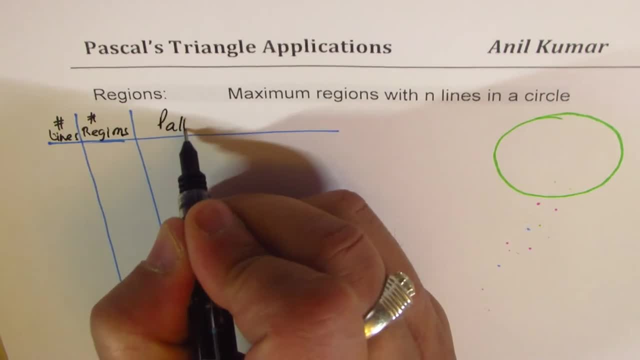 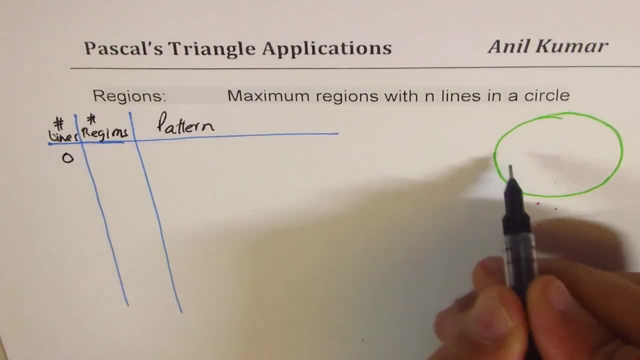 correct and we'll recognize some pattern to fit in the formula. that's the whole idea. so if the number of lines is zero, i mean no lines at all. we have one region, right? so that is what we have. we've just one number here, so that is with no lines. but suppose if i draw a line here, 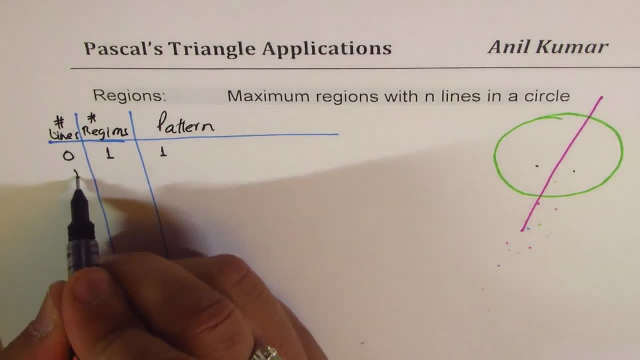 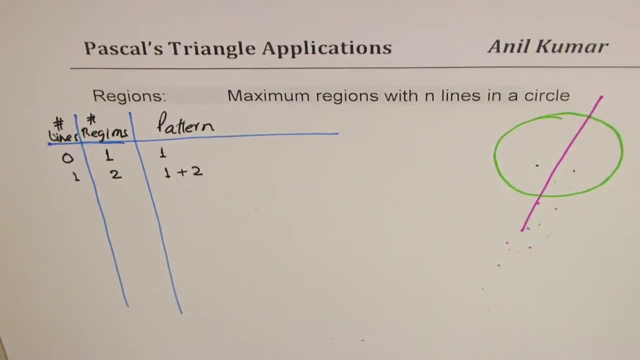 in that case we have two different regions, right? so one line will give me two regions. so what i did was that i added one region with the help of this line. does make sense to you now, if i draw another line here, what really happens? we can count one, two, three, four. so with two lines, 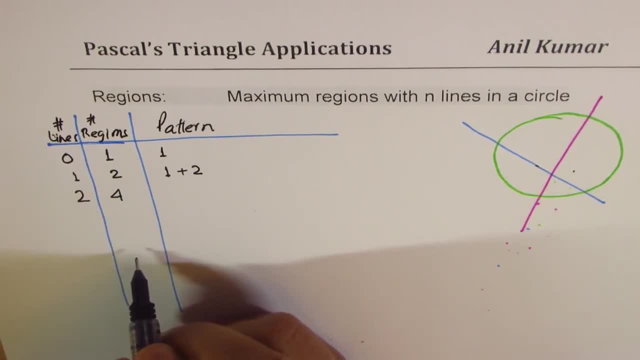 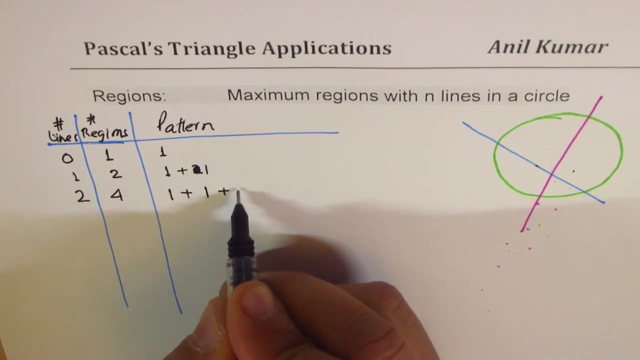 we have four regions right now. what has really happened here is that i mean, this was one plus one. i'm sorry, two is one plus one. so what happened really is: with this line, i actually added two more regions, so additional one more. do you see that pattern going up? 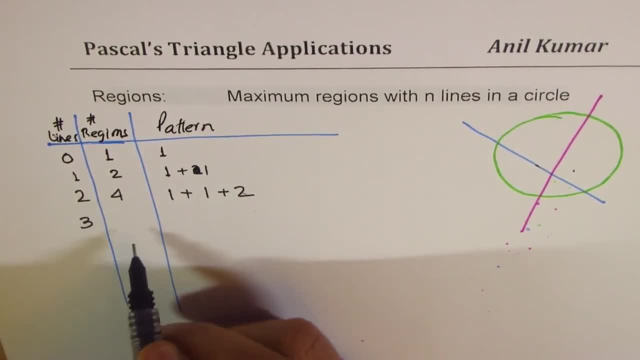 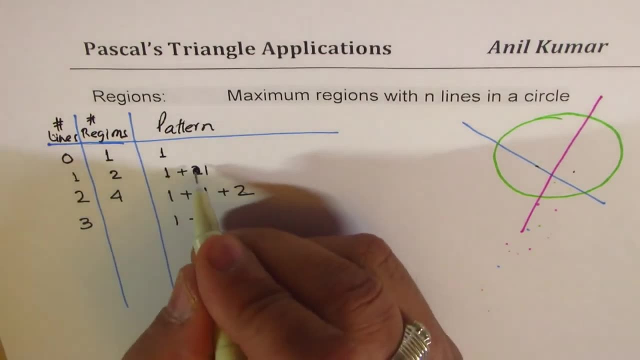 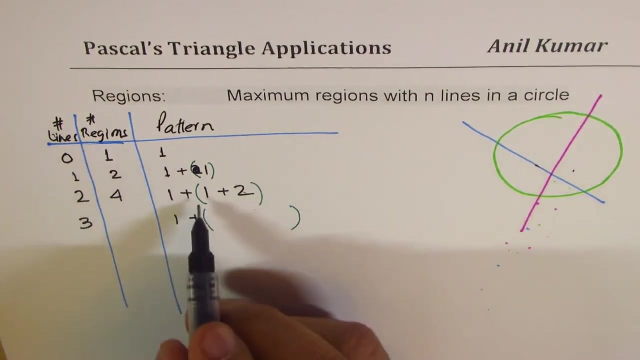 correct. so for the, for the third line, i should get how many? if i look into the pattern which i am going to see, like this one is initially there. i am adding these numbers, do you see that? so what should i do? so we added one plus two with another line. 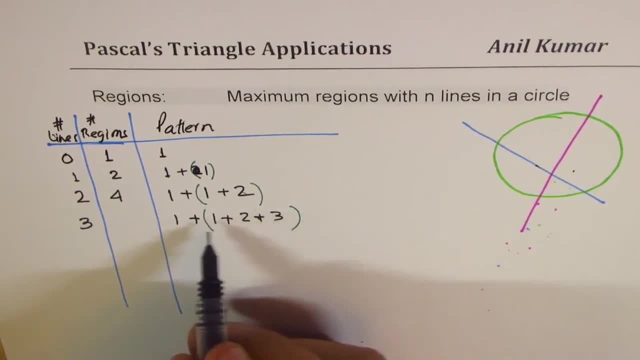 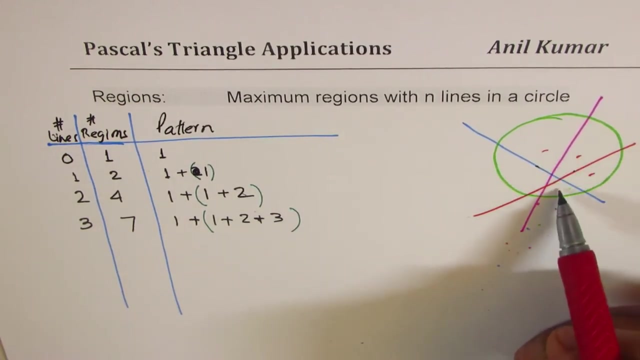 we are going to add three and when you add these terms you actually get the number seven. here we are talking about maximum regions, remember that part, right? so then, one, two, three, four, five, six, seven. do you see that we have seven regions correct? so, because i've actually taken this part very small, i'll not continue further drawing and 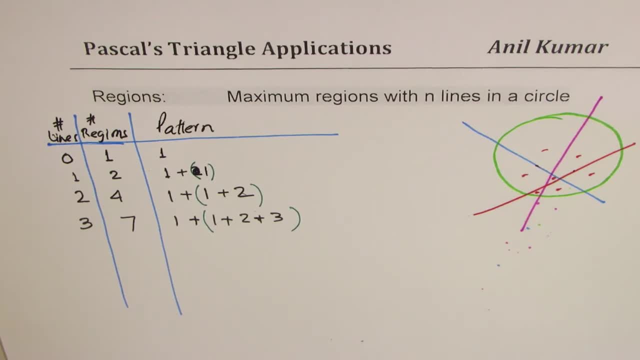 showing you the lines, but i hope you get the concept. that is the maximum number of regions you could get, right. so with the next line, in addition, we'll get four more regions. so 4 plus 7 gives you 11, right, so we get 11. and here you can see the pattern, this sum of natural numbers. 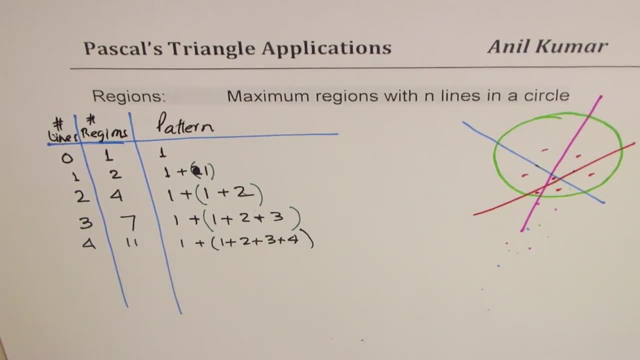 do you see that part right? it is sum of natural numbers. and does that remind you of something? now, sum of natural numbers in your patterns is given by the second diagonal right. this is the second diagonal which gives you sum of natural numbers. perfect, that is the second diagonal. so what do i do? 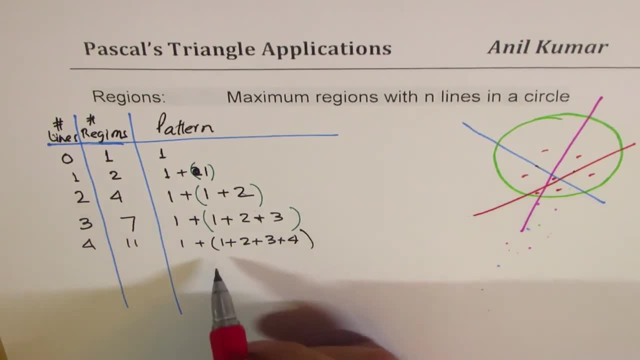 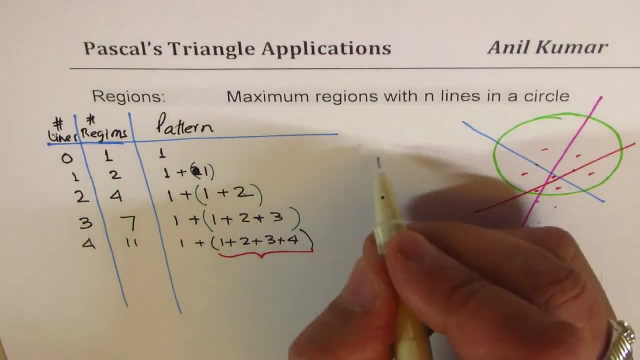 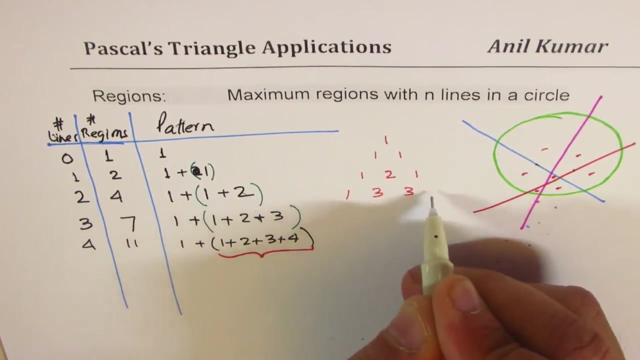 i do. so what does that mean? i have to count, i am going to say these without a muscle and i don't have to type. we see here is okay. let me quickly make this and then you will see for yourselves. it's easy to make the diagonals and we need practice correct. so that's what we are doing here. for some of you, 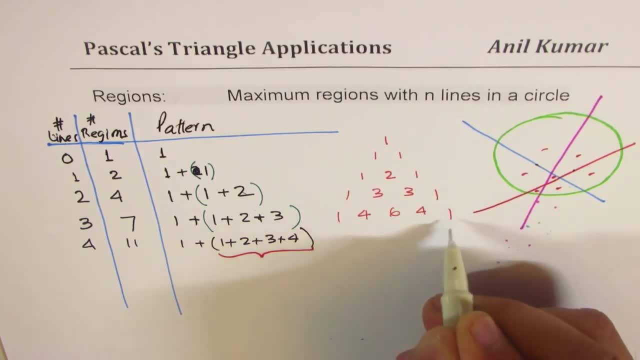 this may be a new thing. I hope you enjoy making all these and also understanding the concepts right. it is helpful and easy to explain. that's why I'm taking some time. we'll just add this: this be 15, okay, and then this be 20, and this is 20, and this is 6 and this is 1, okay, so likewise we can. 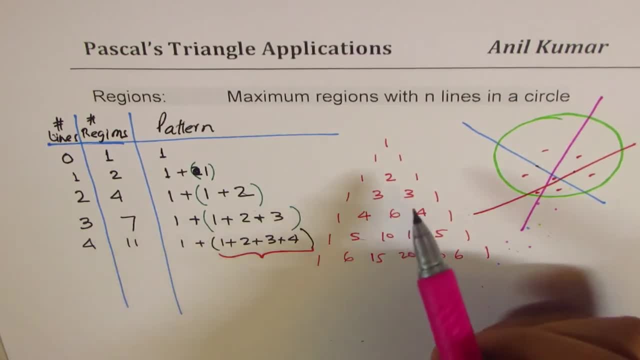 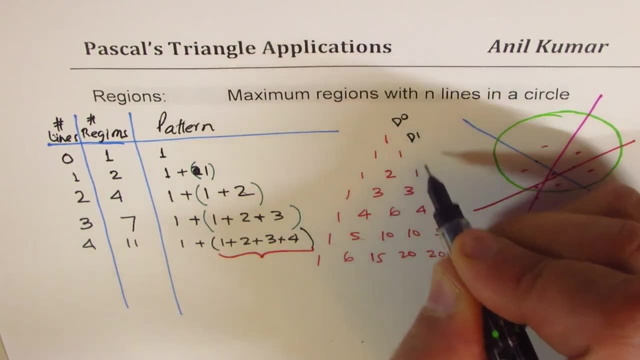 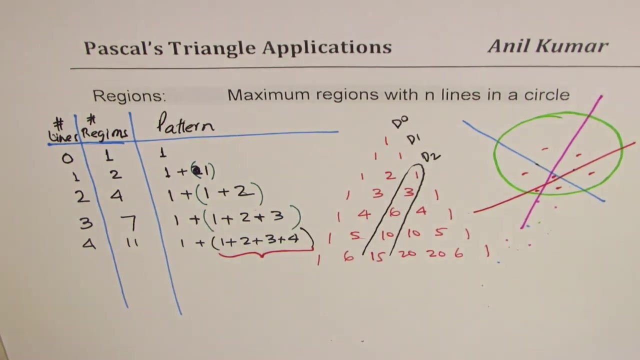 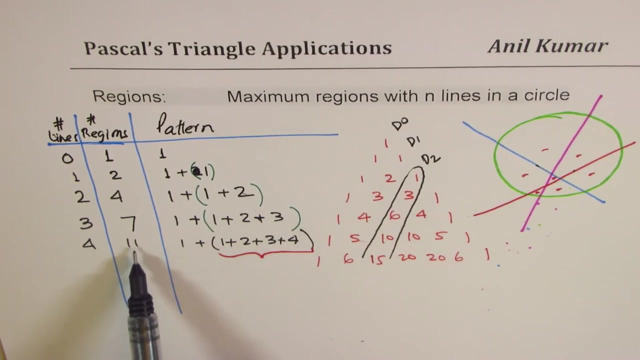 go second diagonal which we are talking about. this is diagonal 0. right, this is diagonal 0. let me write D 0. this is diagonal 1. this is your diagonal 2, so we're talking about this tag. so it is 1 plus 1. 2 plus 1 is 3 and this number is 6, right? 1 plus 10. do you see that number, so that 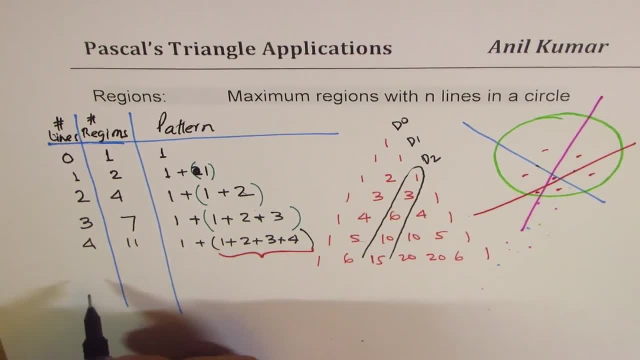 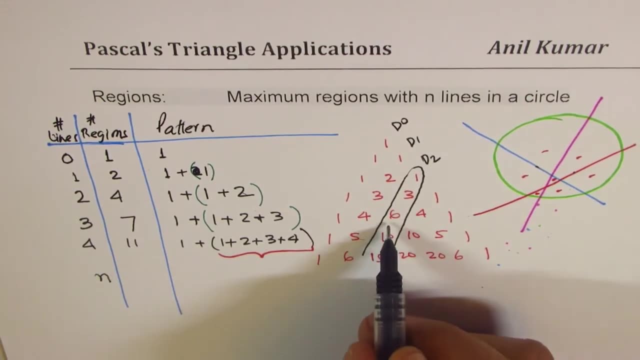 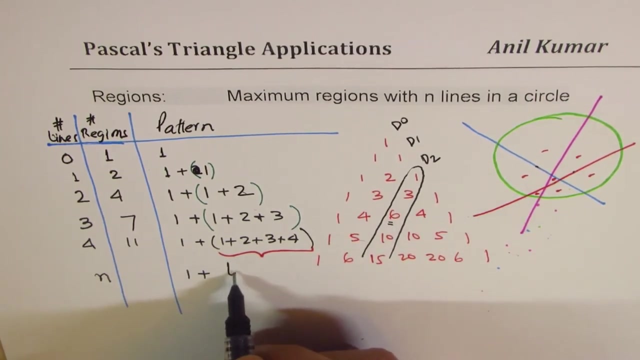 is the second diagonal. so every time if I have nth line here, see, if it was fourth line, then for fourth line we are adding 1 to this position 6, which is t 4, 0, 1, 2. do you get the point? so this is 1 plus t n, 2, does it? 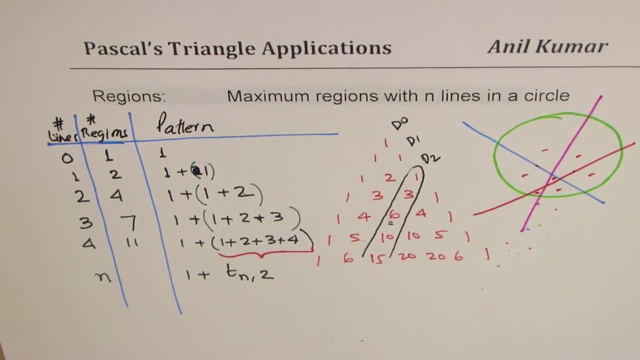 make sense to you. so that becomes your formula, that becomes your formula, and if you really want to calculate without making a long list, you can use combination. so so the rule here is that maximum number of regions, maximum regions with n lines, is equal to 1 plus c, n 2 or n c 2 there. 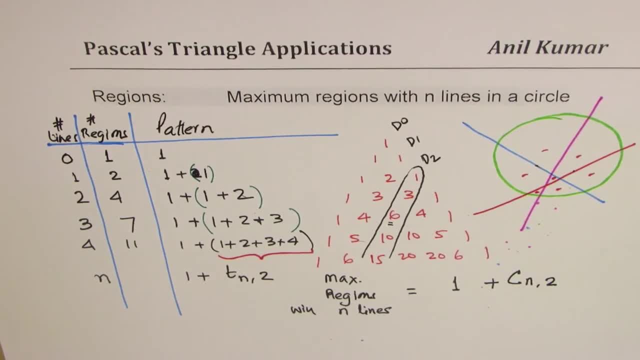 are different ways of writing this. that is your formula, is it okay? you can always use this formula. get your answer perfect. you you can verify with these examples where, as you know what is c n 2, c n 2 basically is, i could write like this: n factorial over n minus 2 factorial times 2 factorial, since you know that, 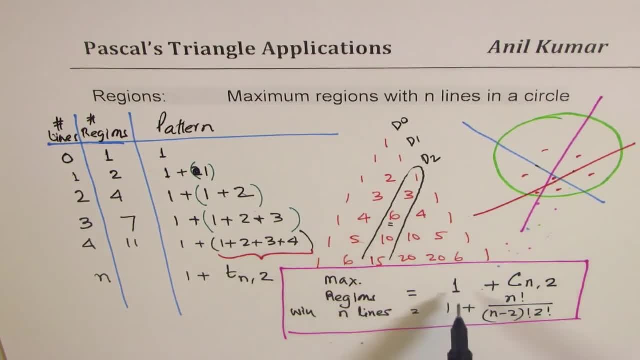 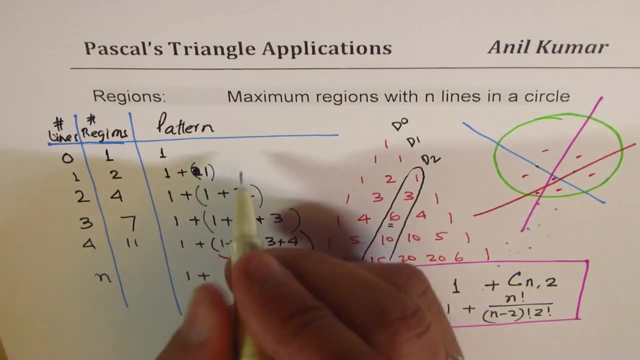 n, c, 2 is sum of natural numbers, right? so you could also write this in sum of natural numbers. this simplifies. to let me write down somewhere here in red ink: okay, that should work. so so you could actually simplify this and write this as 1 plus n times n. 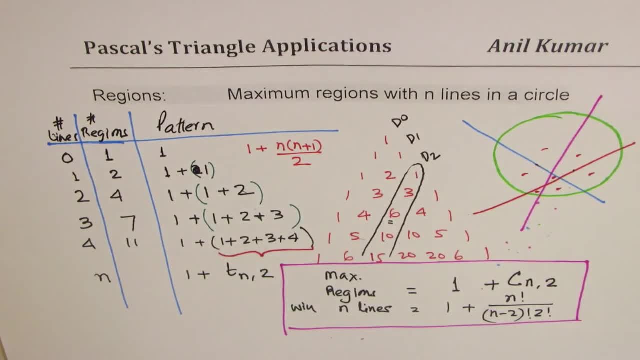 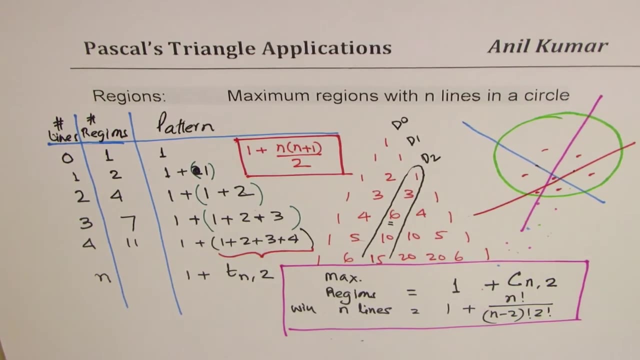 plus 1 divided by 2, which is sum of natural numbers. is it okay? which is this row? so that becomes your answer. but in general, we found it using pascal's triangle, and that is the term number which gives you the number of regions in which a circle can be drawn. so you can. 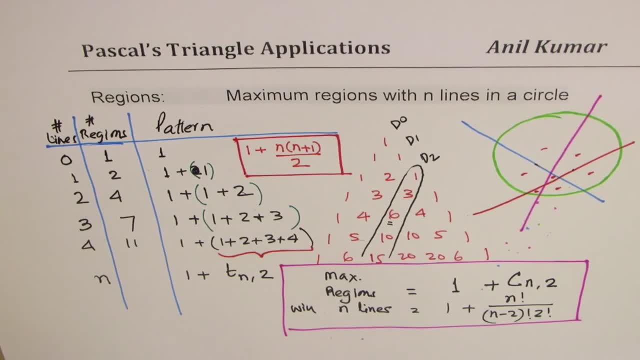 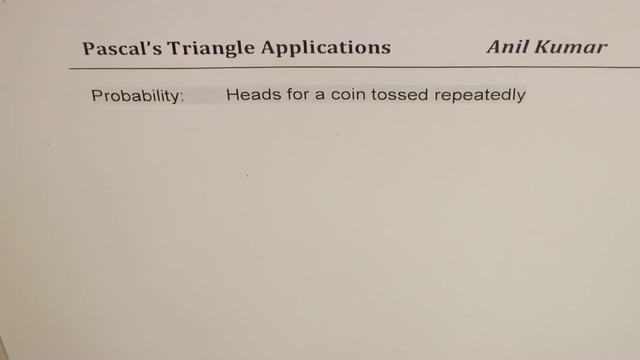 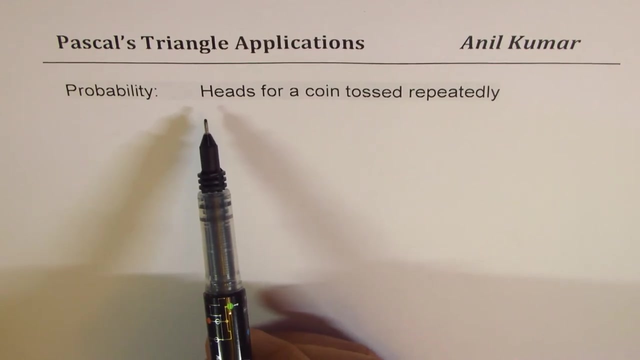 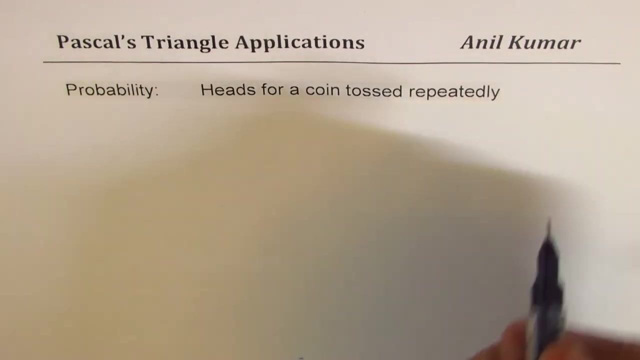 give it what you wanna know. I've done that process all the time. what you can discover is that a total of weiß, die Mitte 1 want I mean direito 4, 15 hours. how do we get a count of heads for a coin which is tossed repeatedly? so, in general, the answer is: 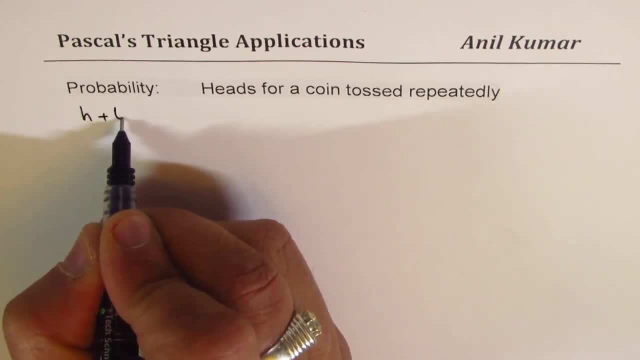 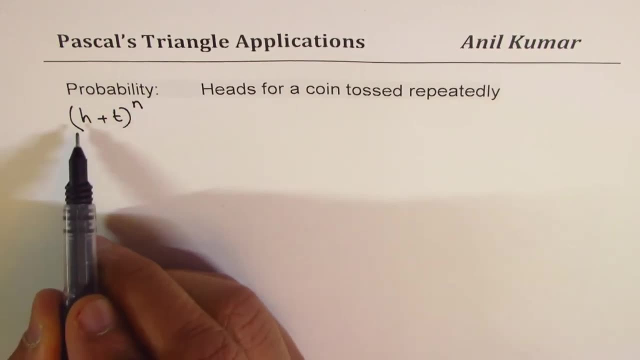 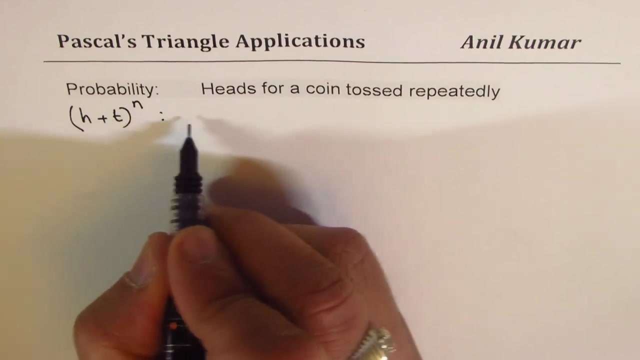 let me write down the answer first. we could use pascal's triangle to answer, and it is: h plus t to the power of n will give you the number of heads when you toss a coin. so if you toss a coin n times, so n times repeated. 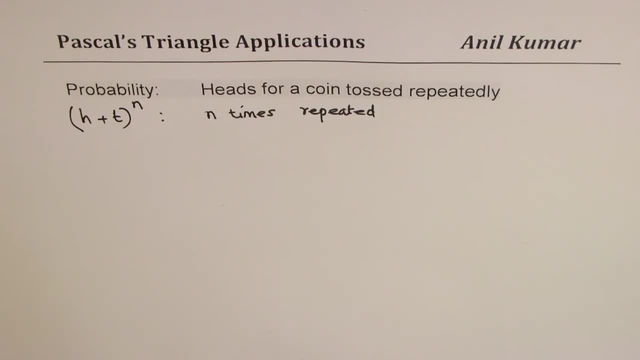 you can find number of heads, or number of tails, for that matter, correct, so that formula will actually help you get the answer. but i've given you the answer. let me give you the logic now. so we are approaching it in a very different way. so i'll take a very simple case. let's assume that 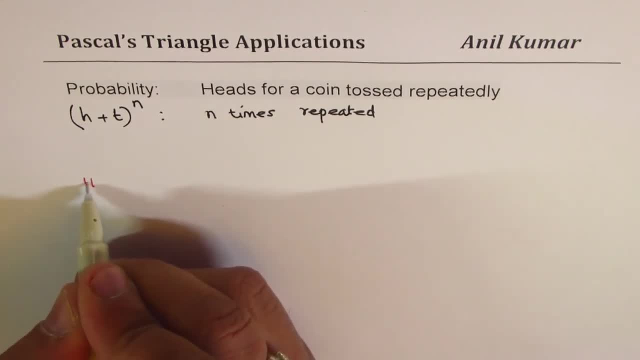 we have a fair coin. so if you toss a fair point, you get either a bunch of heads, or if you have a fair coin, you get a ton of heads. or, for the Microsoft is: just assume that we have a coin e head, or you get a tail. perfect, now, this is in the first toss. next time, if you toss this coin, 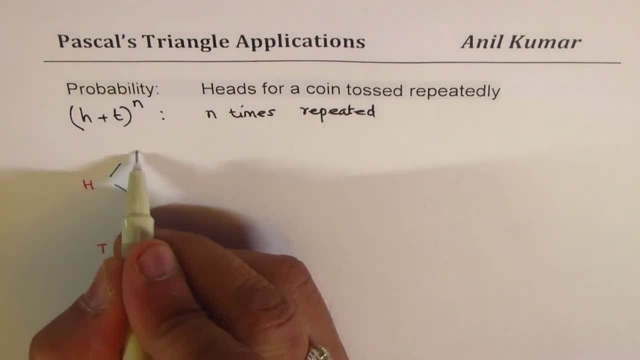 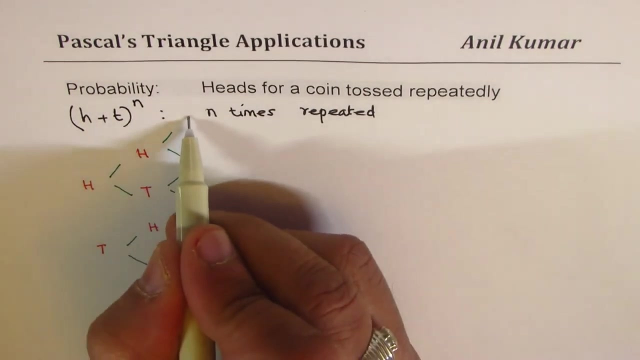 you can again get head or a tail. so we can just build a tree here. you can again get head or a tail- perfect. and if you again toss then then again you can get head or a tail right. so you'll see a pattern which seems to be very similar to what we had been getting using pascal's triangle. 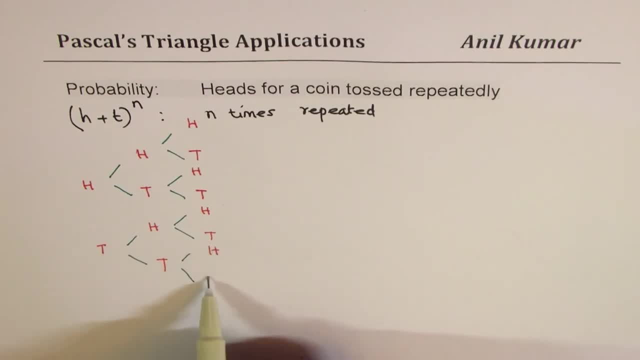 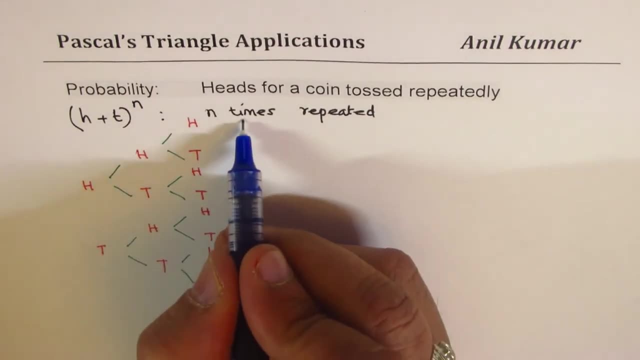 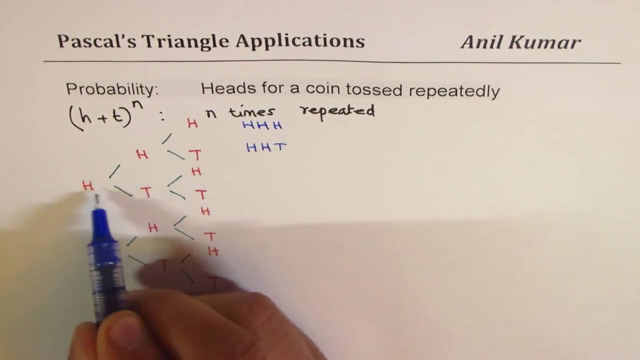 and that is the reason why we can relate these two things perfect. so let's see what we have got. so one way: all heads. so we got all heads here, and then we get head, head, tail, and then we get head, tail, head, and then we get head. 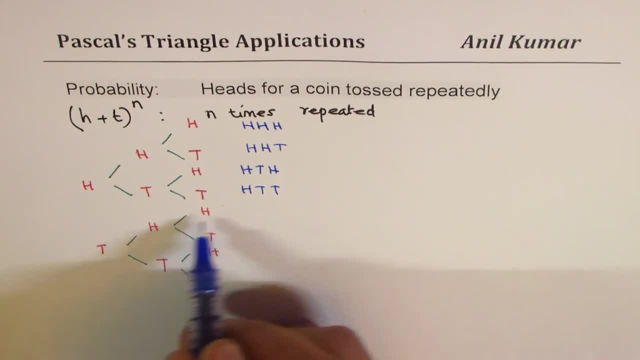 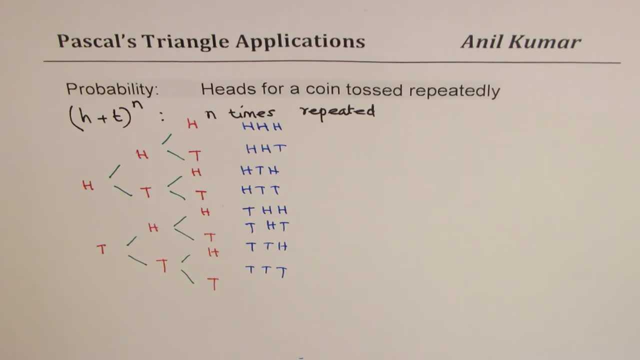 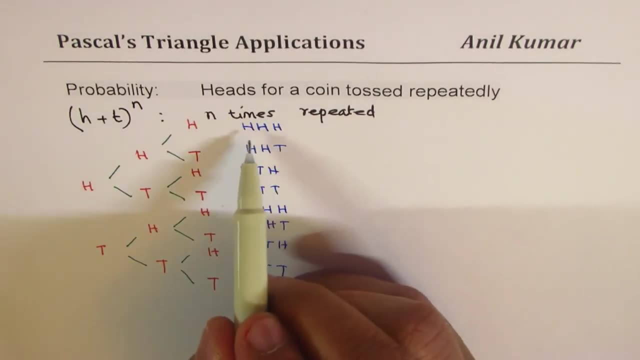 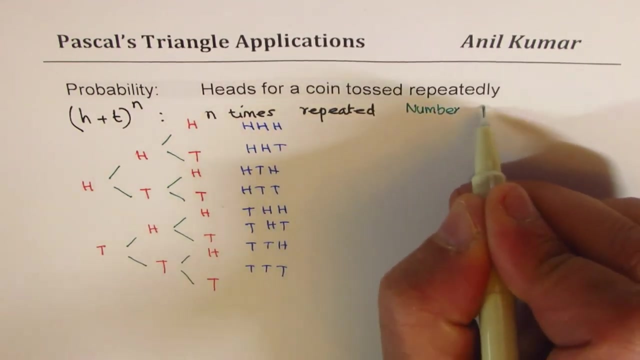 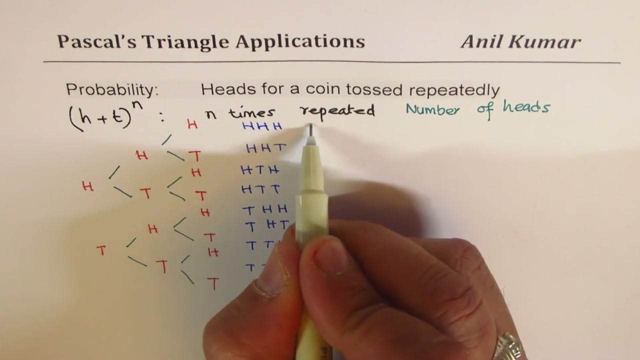 So these are the eight combinations which you can get correct. So what we are also saying here is that you may get we are talking about number of heads, right. So we are talking about number of heads. So the number of heads are three. here let's write: number of heads are three, number of 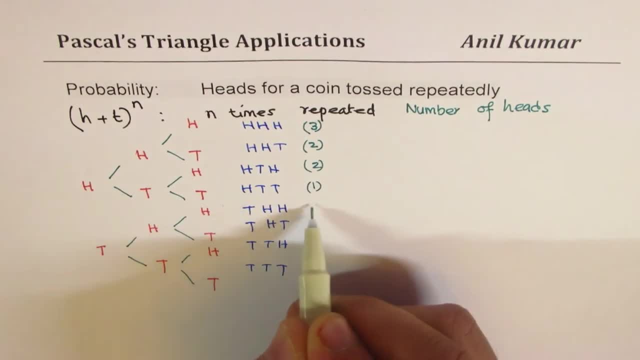 heads are two. number of heads are two. number of heads is one. number of heads is two. it is one here, one here and zero there, correct? So these are my number of heads. Now the question is, in how many ways can we get right? 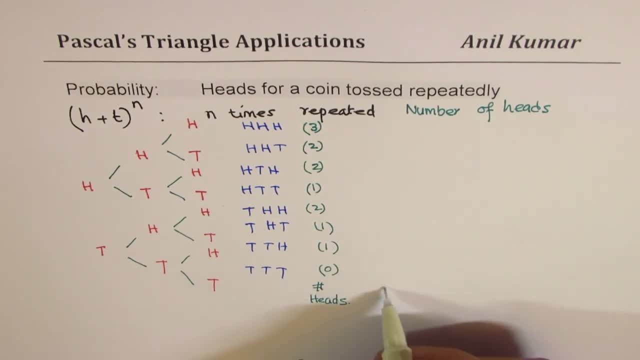 So we have to now figure out in how many ways. So we say number of ways Now. so let's see how many ways do we get three heads, Three heads: you get only one way right. This is taken care of. two heads: one, two, three. 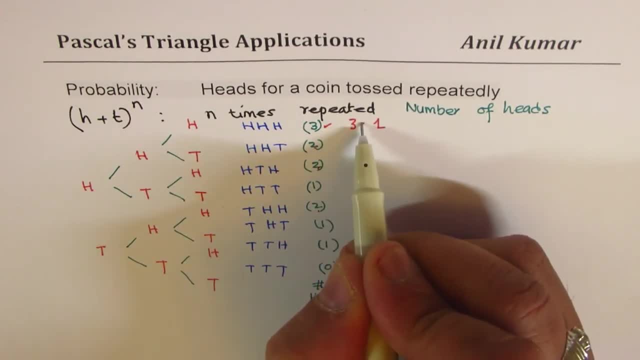 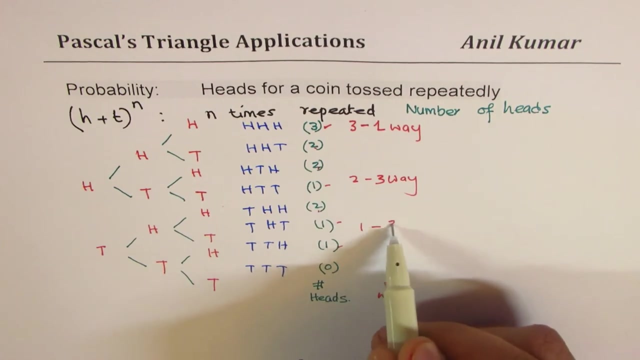 So two heads. let me write this like this: three heads, one way, and then two heads, three ways. right, So three ways. So three ways. one way is it okay. And as far as one is concerned, one, two, three ways and zero heads you could get is: 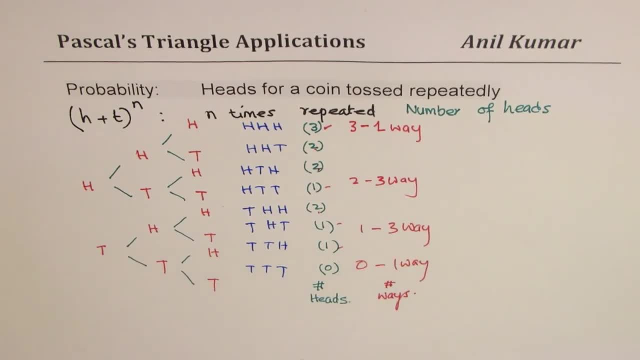 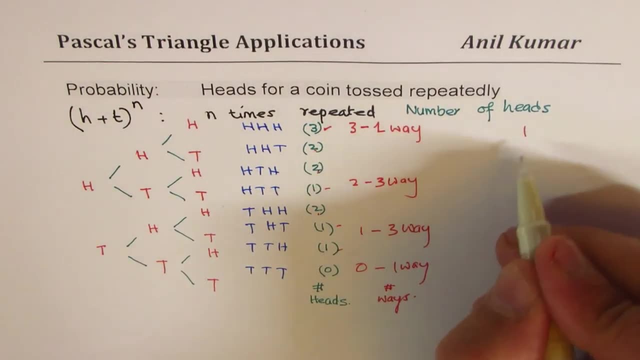 actually one way right. So that's what you get. Now, if I build up the Pascal's triangle, does it all combine. So we have the simple Pascal's triangle, right. So one one and then again one one, and in between you get two here. 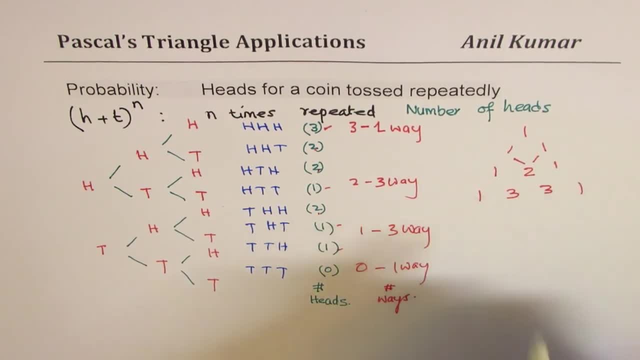 And third row. we get this So, because n I've taken as three, I could say head plus tail to the power of three is equal to what. So that is the coefficient. So we get h cube plus three h squared t plus that coefficient, three h t squared plus 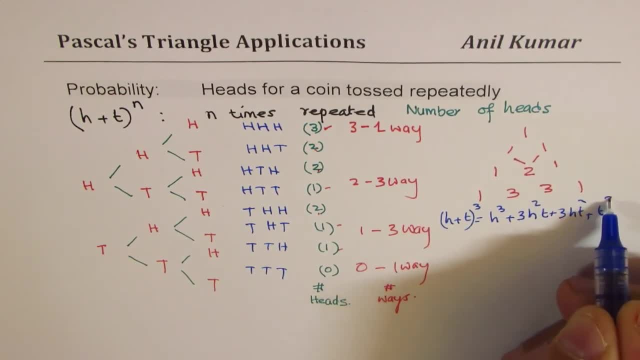 this coefficient And then we get t Q. do you see that? Now, from here it is very clear that if I'm looking for three heads, there is only one way. So this says three heads, one way. Do you see that? 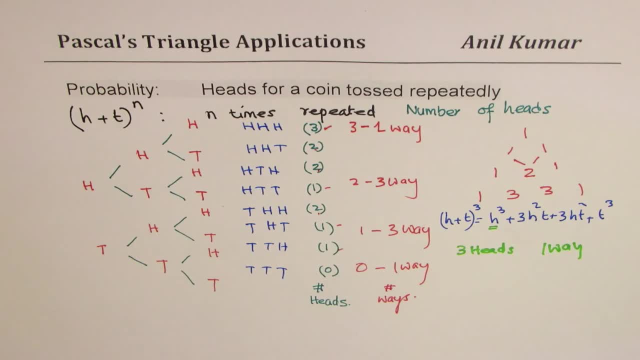 That is what it is saying And the next portion clearly writes down: there are three ways to get two heads. So this is number of heads. So we get two heads. There are three ways. Do you see that? And similarly, you can see that we get three ways to get one head. 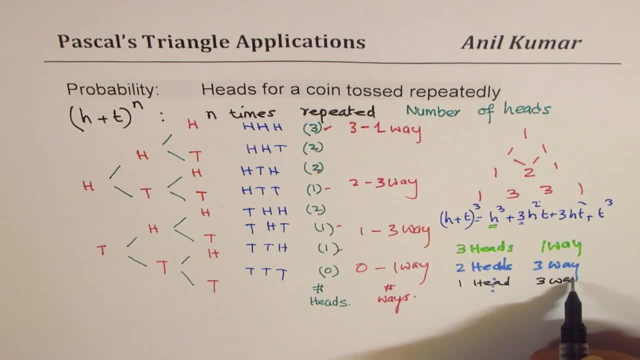 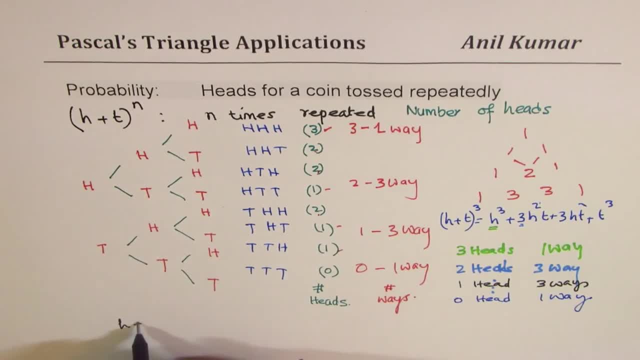 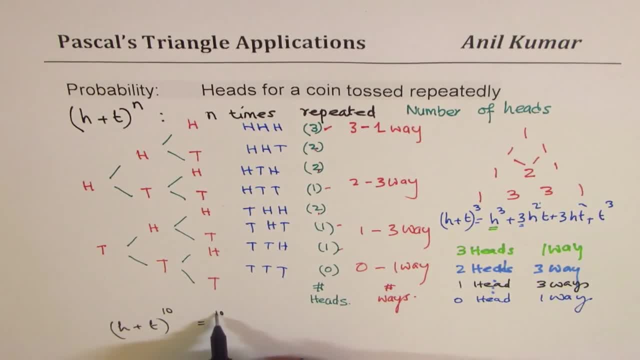 Now it should be 10, I mean normally we write like this: 10C0, right. H to the power of 10 plus C101.. H to the power of 9T1 plus 10T2.. 10 c 2. h to the power of 8 t square. like this you can continue and then at the end you get 10.